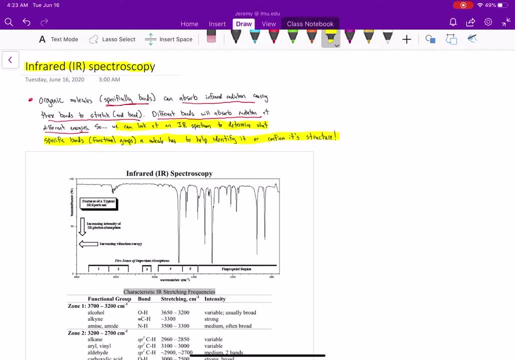 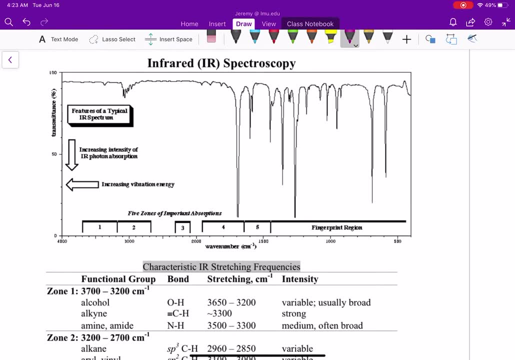 This is the fundamental principle of infrared spectroscopy. So let's look at a typical spectrum here, okay, So if we look at our y axis, we have transmittance right, That's the amount of light that goes through. So the top of the scale we have 100. 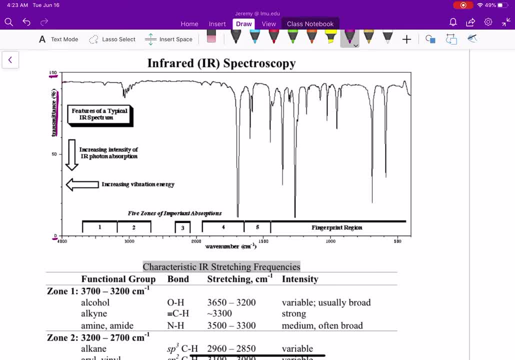 At the bottom we have 0. So if we look at our first signal here, right, we have nearly 100% transmittance. okay, So light is going through our molecule. So what we're most interested in is not looking at when we have 100% transmittance. 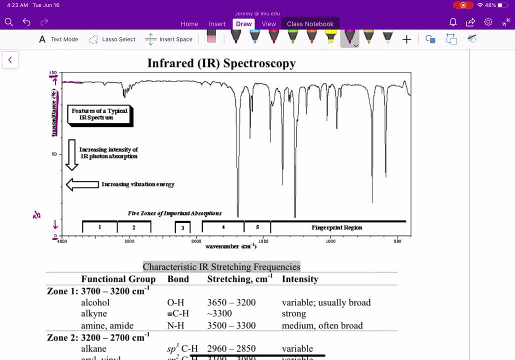 but when we have 0. Transmittance or when we have absorbance, Okay, so we're really looking at identifying peaks. Anytime we see peaks here means that the molecule is absorbing. The molecule is absorbing very specific energy levels, All right. 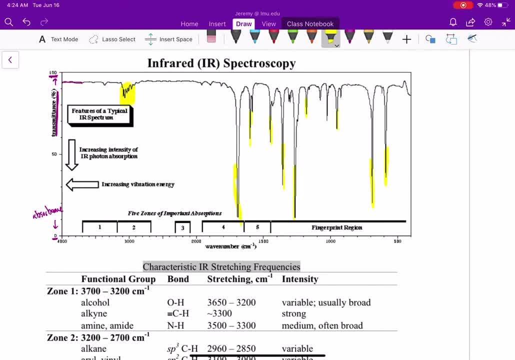 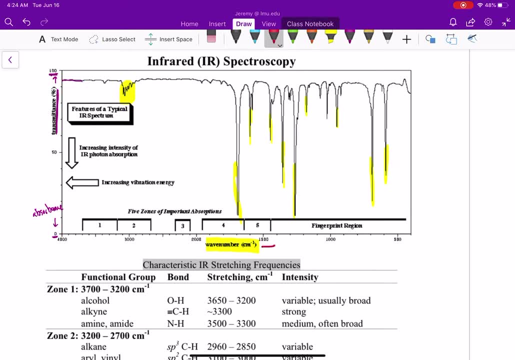 So we're looking at absorbance, All right, Our x axis here is wave number. Okay, So this is just basically a number That really corresponds to our energy. Okay, It corresponds to our energy or our frequency. So here we're just using numbers that are easy for us to work with. 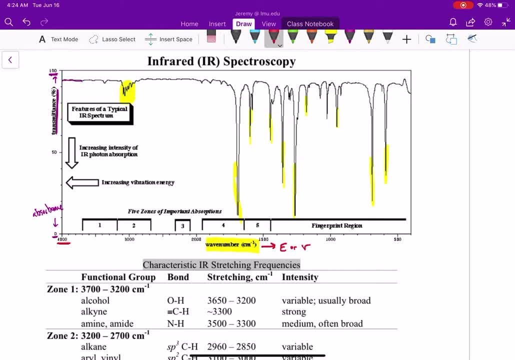 Our general scale is from 4,000 wave numbers to about 500 wave numbers, And the official unit of a wave number is 1 over centimeters. All right, 1 over centimeters. Okay, So you can see that unit here. 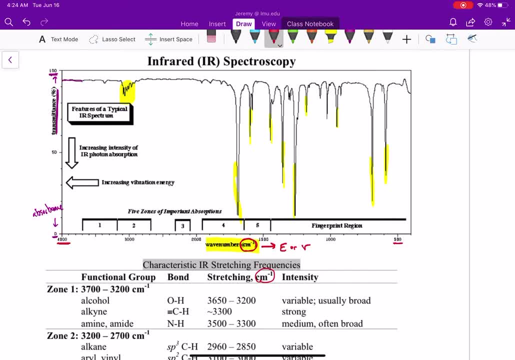 But these are just values that help us to identify where these peaks come. All right, Where these peaks are Okay. So this is what a typical spectrum looks like. We're looking for absorbance. We can see what that intensity is by how large the peak is. 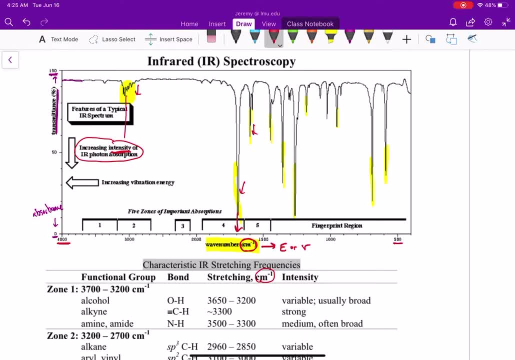 But most important, where these absorb, Where these peaks actually absorb. Okay, So we're going to be looking at these values here on what energy is absorbed. All right, To break this down and simplify it, what I'd like to do is really talk about five different. 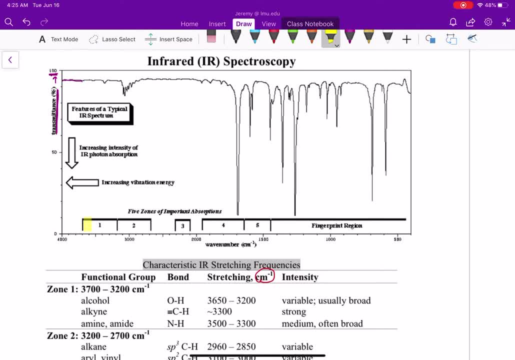 zones. So we're going to be focusing on our attention on five zones: Zone one, zone two, zone three, zone four and zone five. Okay, So these are the five zones that are going to be important where we can see peaks. 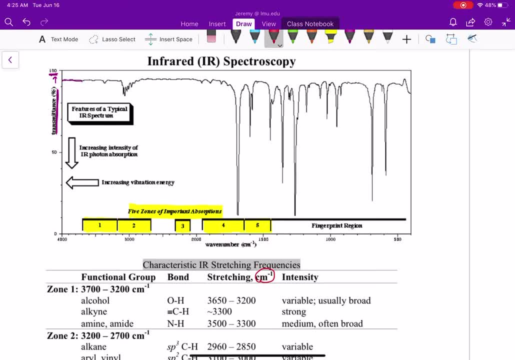 Okay, This last region here is called the fingerprint region. Okay, And we're not really going to be focusing on this region that much, because there's generally a lot of peaks here And these peaks tend to overlap. Okay, So, there's a lot of peaks and they tend to overlap. 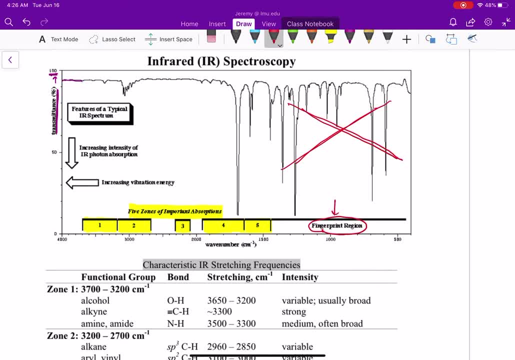 So it's hard to identify a molecule looking at the fingerprint region When we're just learning basic infrared spectroscopy, Right? So what's important is going to be looking at our five zones. Okay, And again we're going to be looking at bonds. 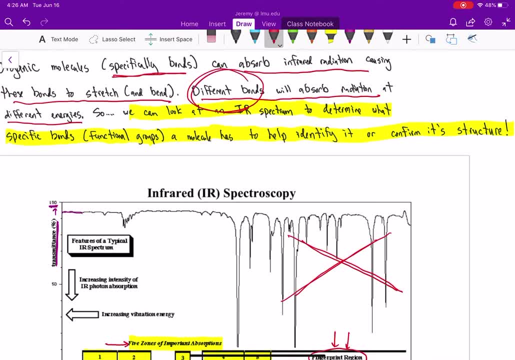 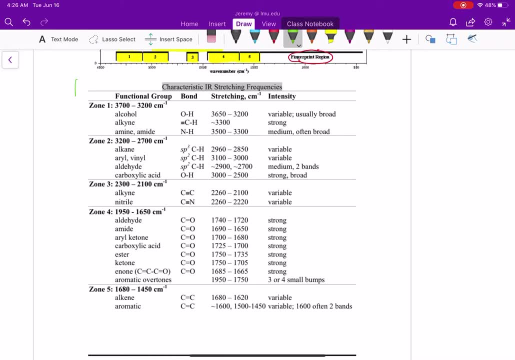 All right. So the first thing we have to do is we really have to look at our table here. This table is going to be very, very important to understanding IR Right. These are our character regions. These are our values. Okay, 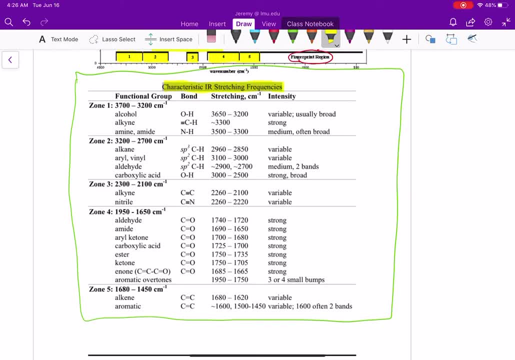 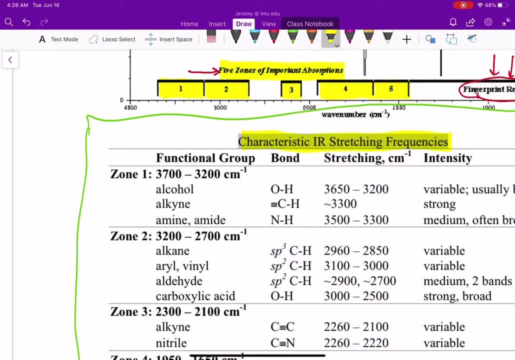 These are our characteristic IR stretching frequencies or energy. All right, So let's break this down into our five zones. So our first zone is zone one. This comes between 3,700 and 3,200 wave numbers. Right One over a centimeter is wave numbers. 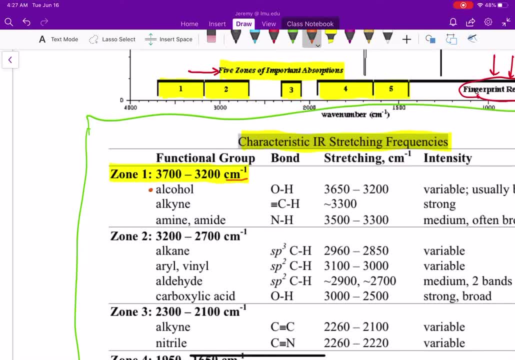 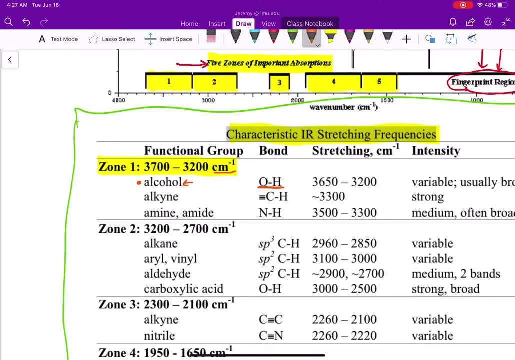 So there's three main functional groups we're going to be looking at. First is an OH bond Right, And that can be found in the functional group of an alcohol. So if your molecule has an OH bond, that means that it will absorb infrared radiation somewhere. 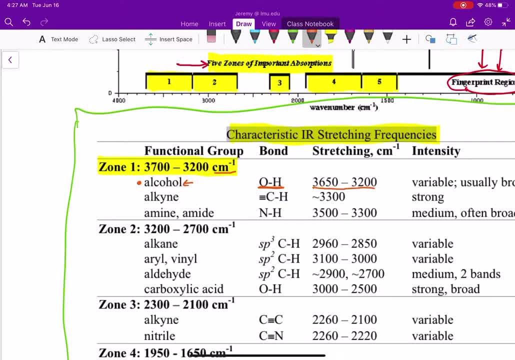 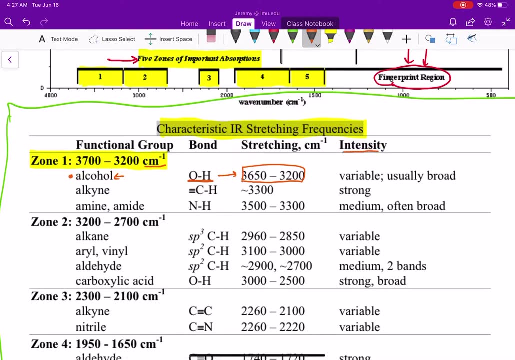 between 3,650 and 3,200 wave numbers. All right, So OH bonds will absorb between 3,650 and 3,200.. And then here we can talk a little bit about the intense intensity. This absorbance is usually going to be broad. 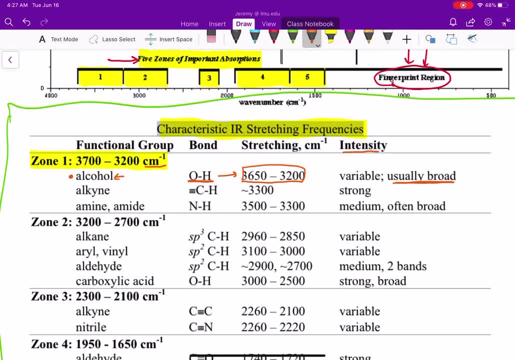 It's not going to generally be a sharp peak and it's usually pretty strong. It says variable here, but generally those are pretty obvious and pretty strong. So that's the first bond we need to look at. The second bond we need to look at is an alkyne, but not the carbon-carbon triple bond. 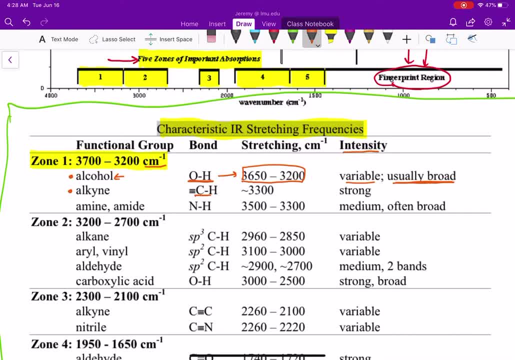 We're actually specifically looking at the sp carbon to H. So we're looking at an sp carbon to H bond, Okay, And an sp carbon to H bond will absorb at about 3,300 wave numbers And generally that's going to be quite strong. 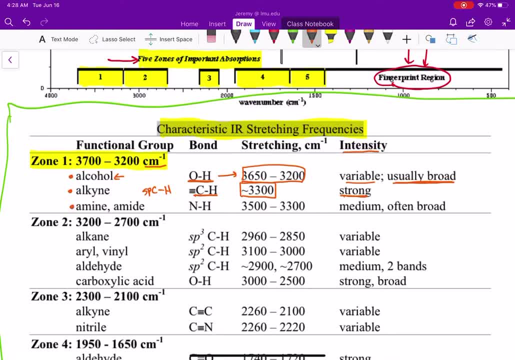 The last bond we need to look at is an NH bond that can be found in amines or amines, So an NH bond will absorb in this same zone and that will absorb between 3,500 and 3,300 wave numbers. 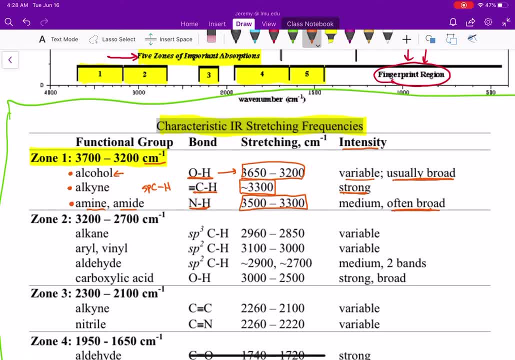 And again, those are often broad. Okay, So in zone one there's three bonds. we'll be looking for An OH, sp, carbon to H and an NH, And they can come at the wave numbers shown here. All right, 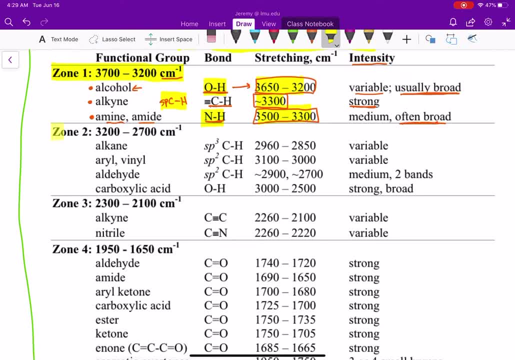 Next is zone two. Zone two is from 3,200 to 2,700 wave numbers. Okay, There's really four groups we need to look at. First is an sp3.. C to H bond That can come between 2,960 and 2,850. 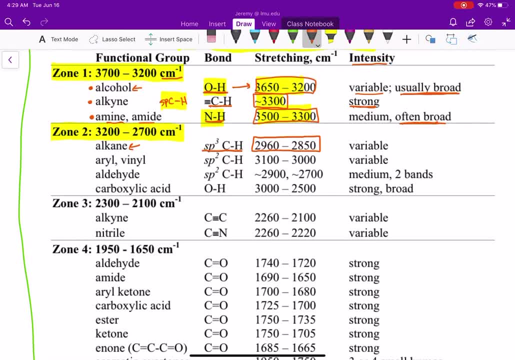 Right, That would be an alkane functional group. All right. Next is aryl or a vinyl. That's an sp2, carbon to hydrogen. That can come between 3,100 and 3,000 wave numbers And you'll see both of these. the intensities can be variable. 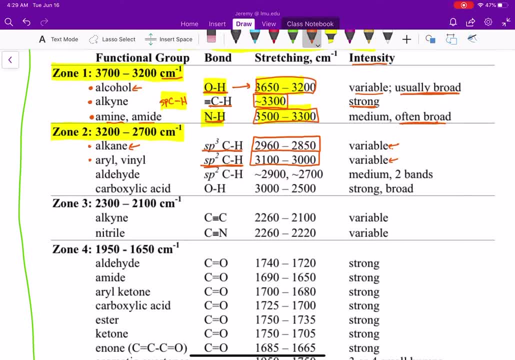 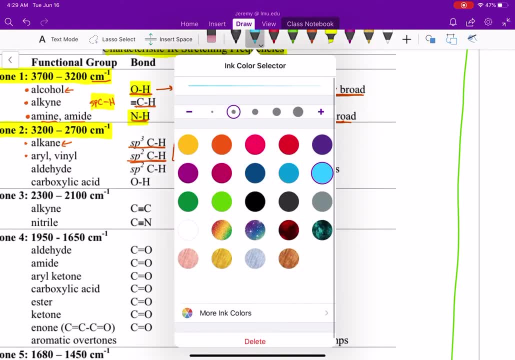 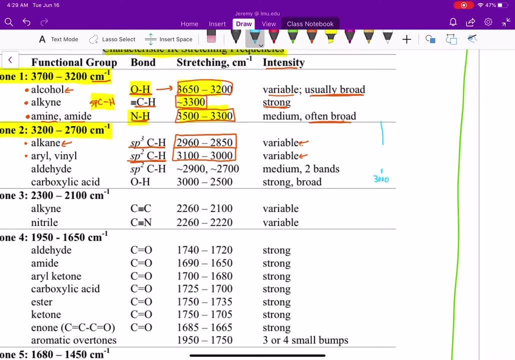 Sometimes these peaks are very intense, Other times they can be small. All right, And to help distinguish these, I like to look at what I call the 3,000 line. So anytime I'm looking at a spectrum, I'll look at the mark for 3,000 and I'll draw a line straight up here. 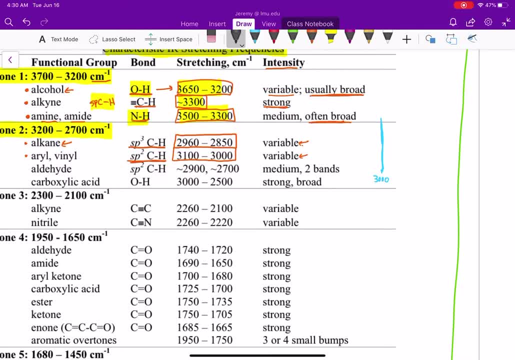 Right. So if I see peaks to the left of this line, from 3,100 to 3,000, these are going to be my sp2- carbon to hydrogens- And if I see peaks to the right of the line from 3,000 to 2,850.. 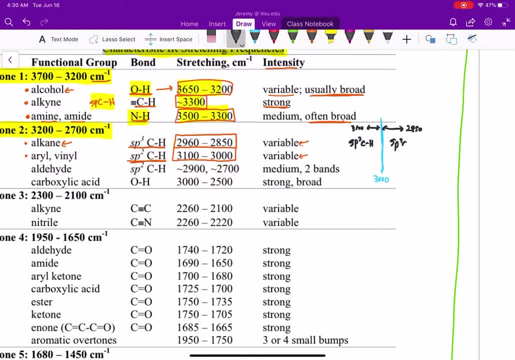 Right, These are going to be my sp3 C to Hs Right. And as you can imagine, in organic chemistry we have a lot of sp3- carbon to hydrogens. So it's kind of be it's generally going to be rare for us not to see a peak there. 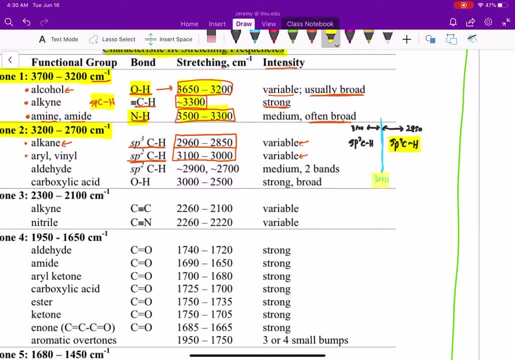 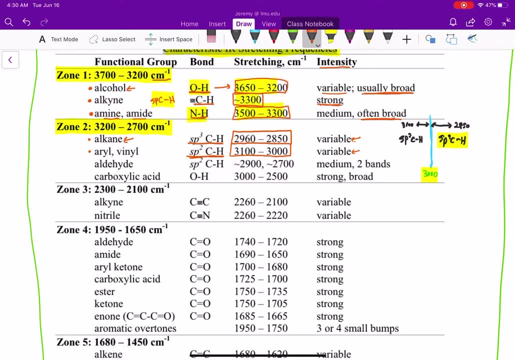 All right. So that's what I like to call the 3,000 line, And as we're seeing spectra, you'll see me draw that in a lot. Next is an important peak, an aldehyde peak. This is the sp2 C to H bond. 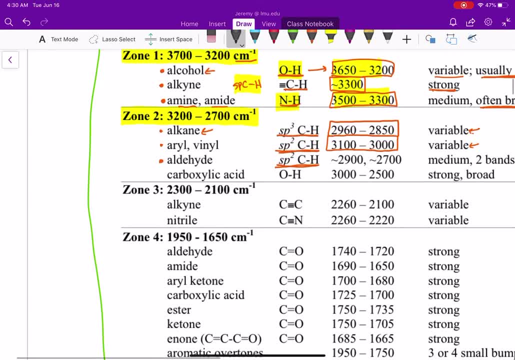 So let's kind of draw that out here. So if you remember the aldehyde functional group, we're specifically looking at the sp2 carbon to hydrogen bond, Right, We're looking at this bond right here. So that bond will have two peaks: one peak at 2,900. 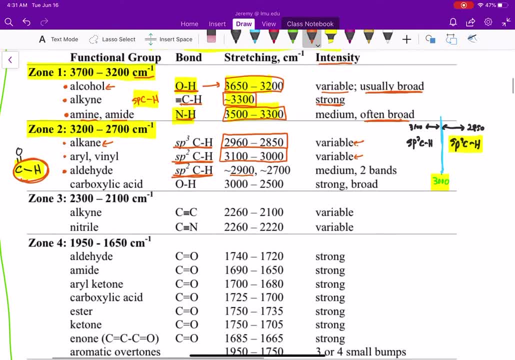 But you'll see that peak at 2,900 is generally going to be kind of hidden in our sp3 C to Hs Okay. So the 2,900 peak is a little hard to see, But what isn't hard to see is that peak at 2,700.. 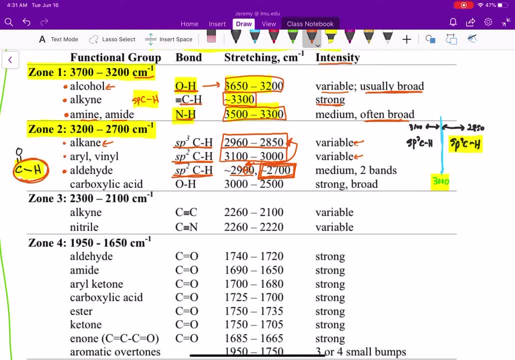 Okay, Nothing else absorbs at 2,700.. So if you see a peak at 2,700, that's telling you that you have an aldehyde functional group, All right. And the last bond or last functional group we need to look at is an OH. 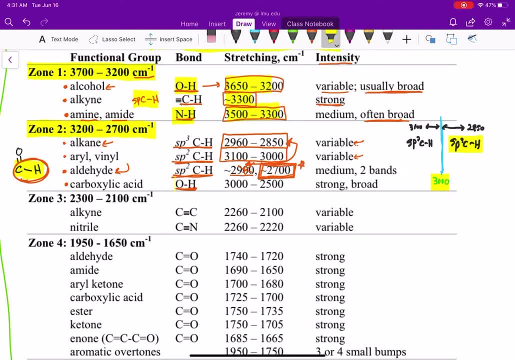 But this isn't any general OH. This is an OH of a carboxylic acid. Notice above: here, an OH of an alcohol is always found in zone 1. But the OH of a carboxylic acid is found in zone 2.. 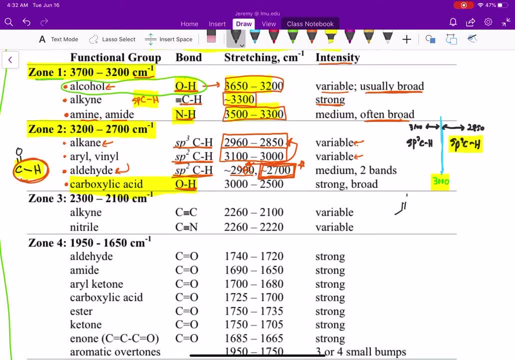 So if we draw out our carboxylic acid functional group here, this OH peak of a carboxylic acid right, this bond here is found in zone 2.. Okay, So that's an important distinction And that will be from 3,000 to 2,500.. 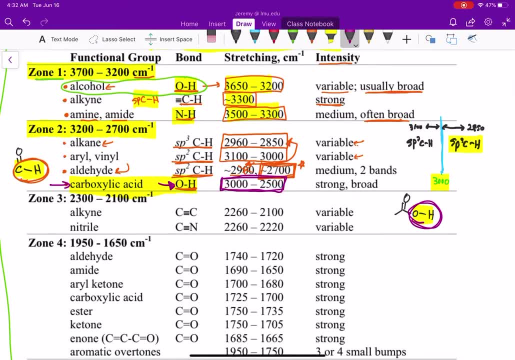 Okay, So again, these are overlapping with some of these other peaks. But what's easy- it's easy to identify these- the OH peaks- is because they are very, very broad. The other peaks we see are generally going to be sharp. 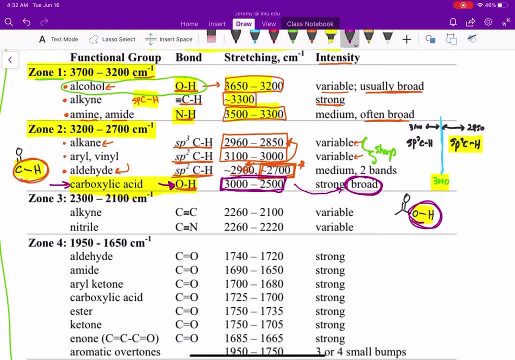 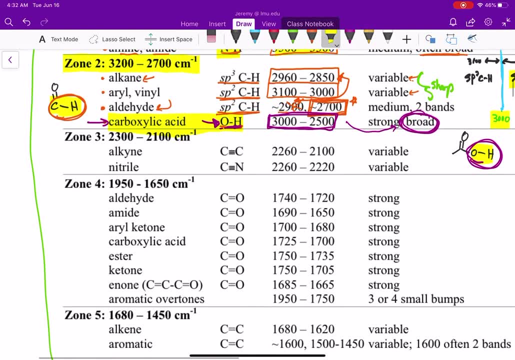 They'll be very distinct peaks, But that OH of the carboxylic acid, that's going to be a broad peak. All right. The next zone we're going to look at is zone 3.. That comes between 2,300 and 2,100.. 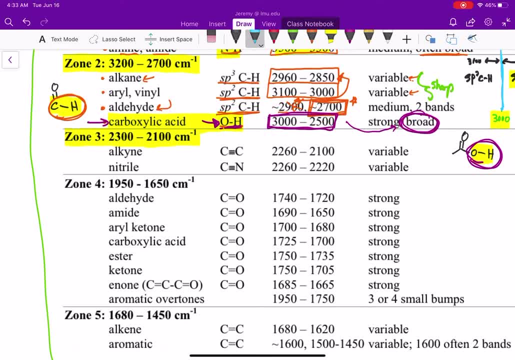 And these are going to be our triple bonds. So my carbon-carbon triple bond or a carbon-triple bond to an N. So a carbon-carbon triple bond is between 2,260 and 2,100.. A carbon-triple bond N is between 2,260 and 2,200. 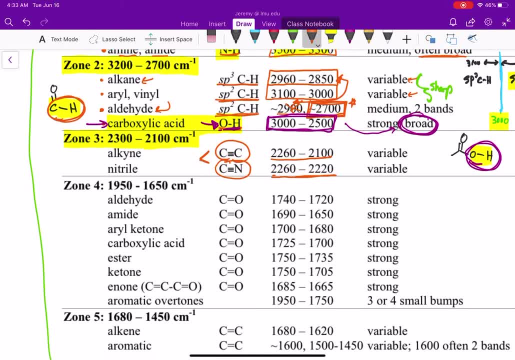 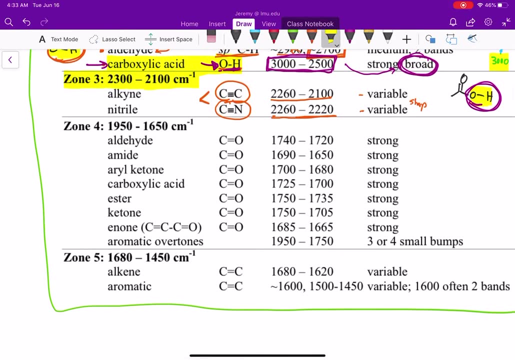 Okay, So our triple bonds are found in zone 3.. Okay, No triple bond, no peak in zone 3.. These both have variable lengths, but they are generally sharp. Okay, Our next zone is zone 4.. That comes between 1,950 and 1,650. 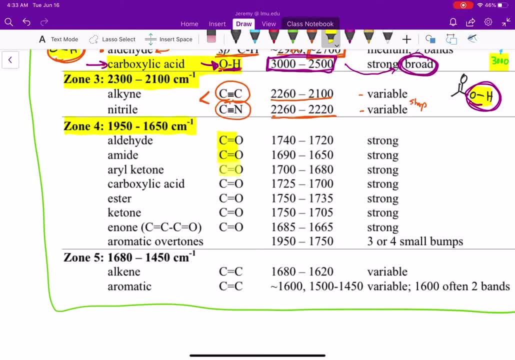 And you can see there's a lot of common things. we have Carbonyls. Okay, Carbonyls can be found in lots of functional groups. Aldehydes have carbonyls. Amides, ketones, carboxylic acids, esters, enones, conjugated systems. 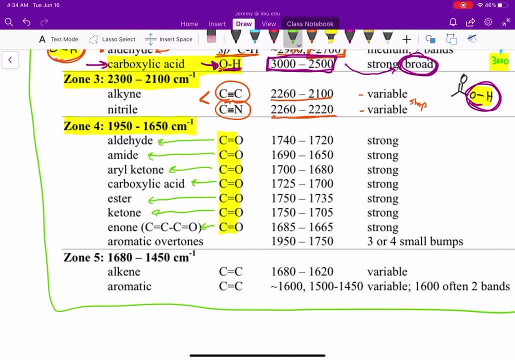 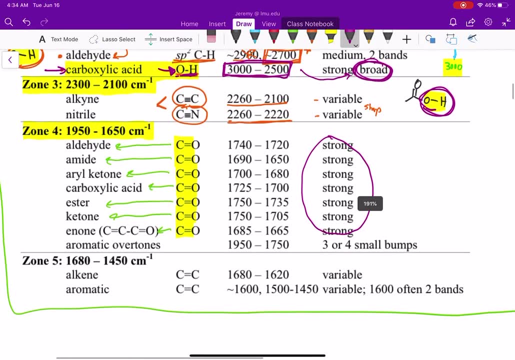 These are all going to be found in zone 4.. I want you to notice all of these are going to be very, very strong peaks. It will be obvious that you have a carbonyl And in my class, in generally speaking, here we can just combine these right. 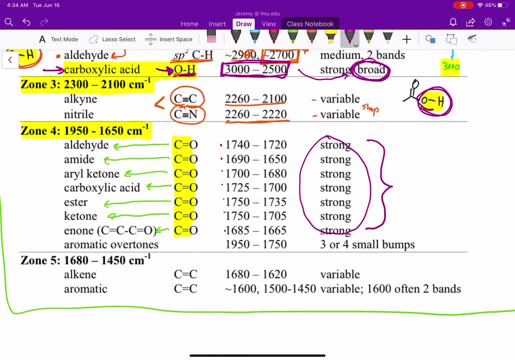 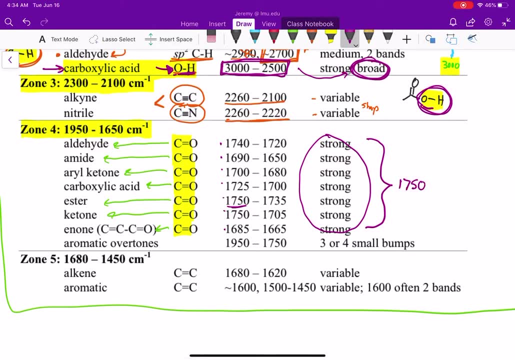 I don't need to separate these out to get specific, because there's a lot of overlap. So, generally speaking, if we see a peak from 1,750 to about 1,680, right, We know these enones can be a little less than that. 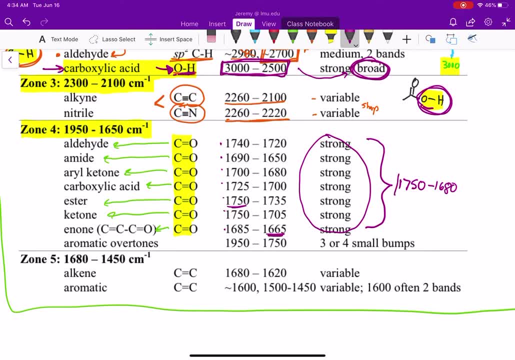 A conjugated can be a little less, But generally speaking, a peak from 1,750 to 1,680 is going to be a carbonyl peak. All right, So all of these are carbonyls. There is one additional peaks. we see aromatic overtones. 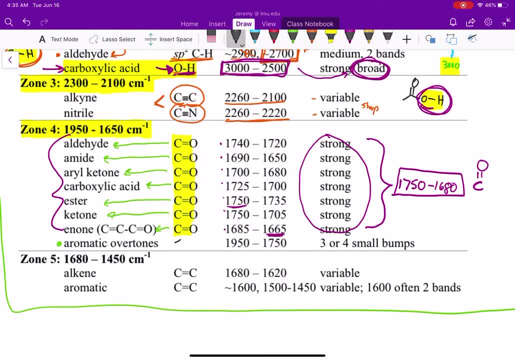 So if you have some aromatic compound, generally benzene rings, okay, You will see three or four small bumps. Three or four small bumps between 1,915 and 1,750.. All right, So those are just small little bumps. 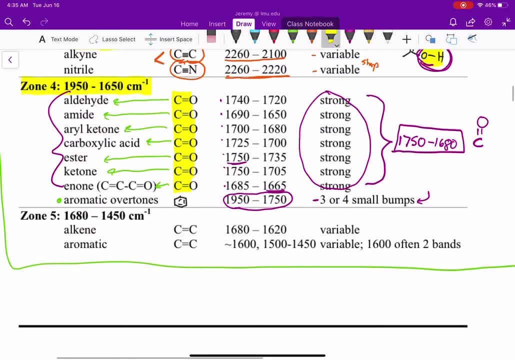 They're not strong. The last zone we need to look at Is zone five. that comes from 1,680 to 1,450.. And these are going to be my double bonds. So a carbon-carbon double bond of an alkene. 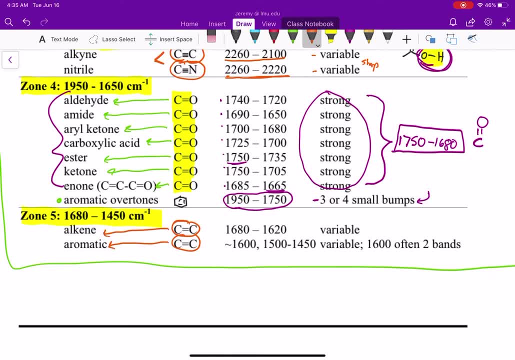 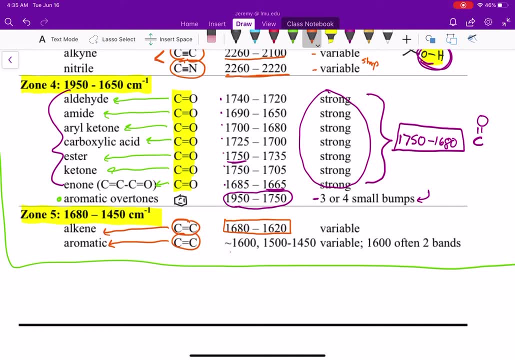 Or a carbon-carbon double bond of an aromatic compound. Alkenes are generally between 1,680 and 1,620.. Aromatic compounds generally will have a peak at 1,600.. And then another peak between 1,500 and 1,500.. 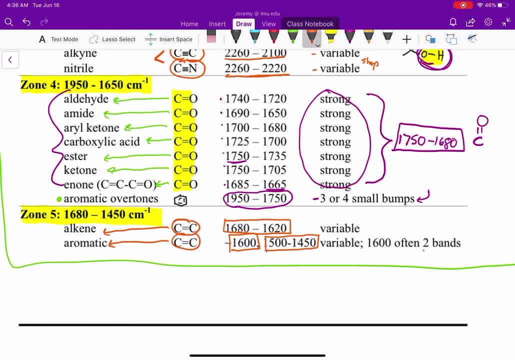 And then another peak between 1,600 and 1,450.. All right, So aromatics generally will have two bands And again, these peaks are generally going to be sharp, Okay, And they can be of variable absorbance, So they can be short or long. 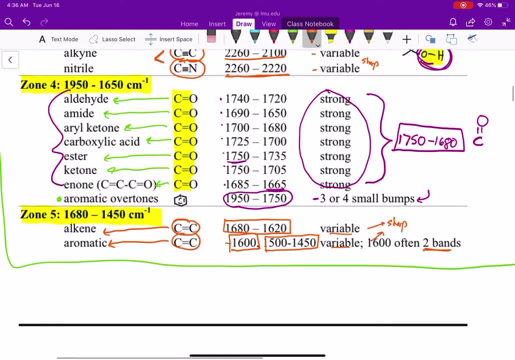 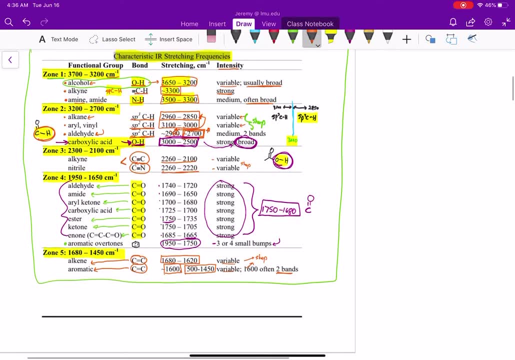 Small or large, But they will definitely be sharp, All right. So these are the main zones that we need to look at and know. What I want to do now is just show you examples of what these actually look like, So I have a lot of sample spectra here. 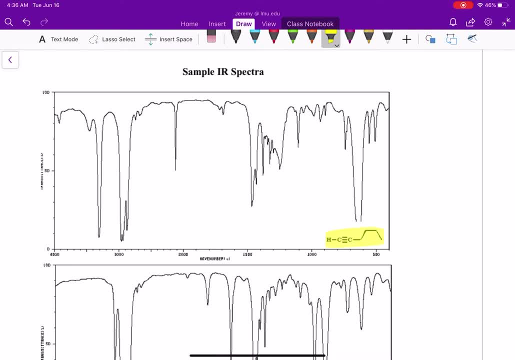 And what you'll notice is in the bottom right corner we have the actual structure. Okay, So what we're going to do is basically analyze the spectrum or the structure to see if we can identify the peaks here. All right, So the first thing we see is, if we look at this peak here I can see a nice big peak. 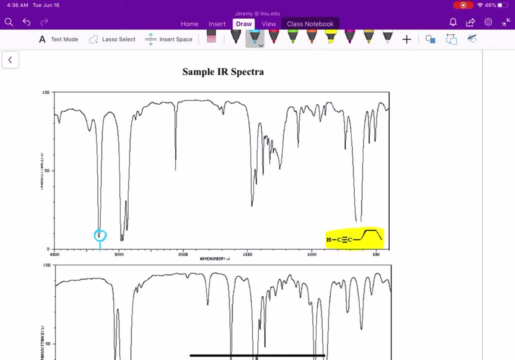 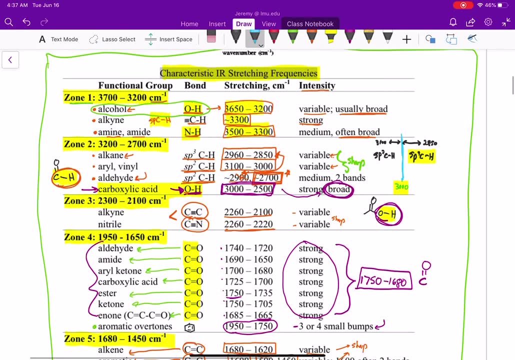 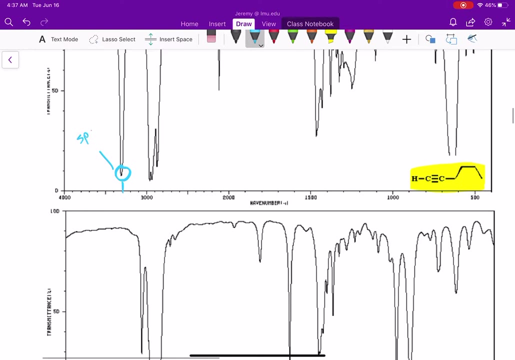 That's at about 3,300.. What does that correspond to? Well, if you go back and look at our table right, a big peak around 3,300 is my SPC to H. Okay, So we can identify this peak as an SP- carbon to H bond. 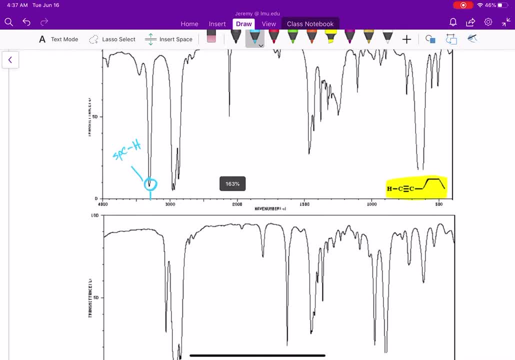 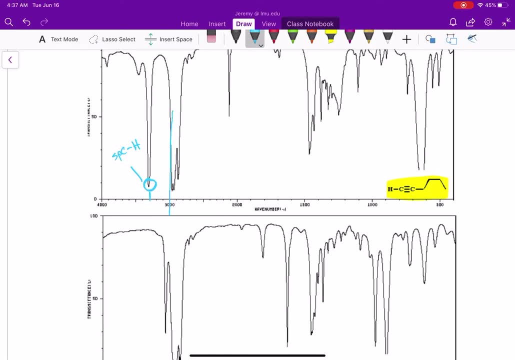 Remember this is always a bond. All right, That's zone 1.. I move into zone 2.. I like to draw in my 3,000 line. There's nothing to the left of this, But I do have a couple of peaks here. 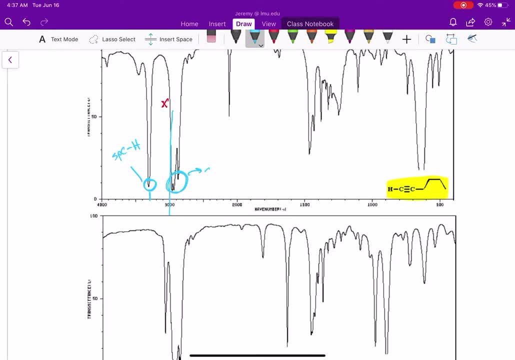 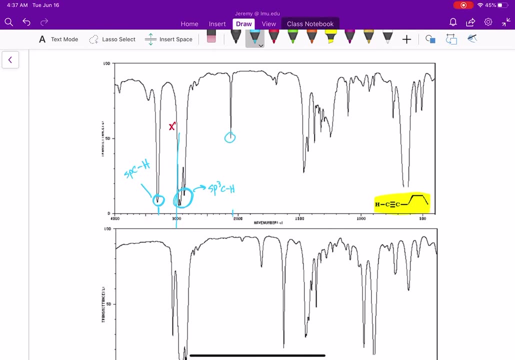 Okay, And those are going to correspond to SP3 C to Hs. Any peak from around 3,000 to 2,850 corresponds to SP3 C to Hs. Next we see a large peak here. That's at about 2,100.. 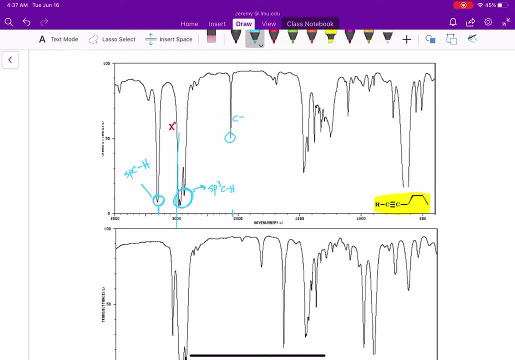 That's where we have our triple bonds. So this is a C triple bond, C Right. This is going to be a C triple bond, N. But obviously here it's going to be a C triple bond, C, All right. And then in my class, once we get kind of below 1,450 or so, we can kind of ignore the rest of these peaks in the fingerprint region. 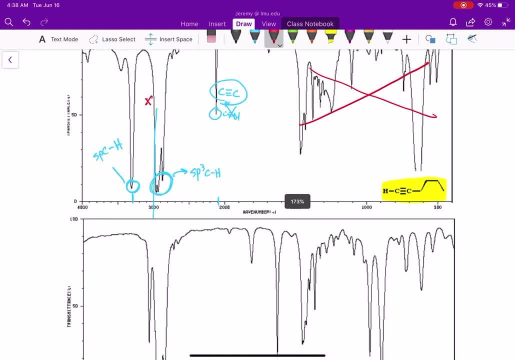 Right. So clearly, what we can see here is we have an alkyne And we have a terminal alkyne, Because I have this SP- carbon to H- right, that's that bond. here I have a terminal alkyne. 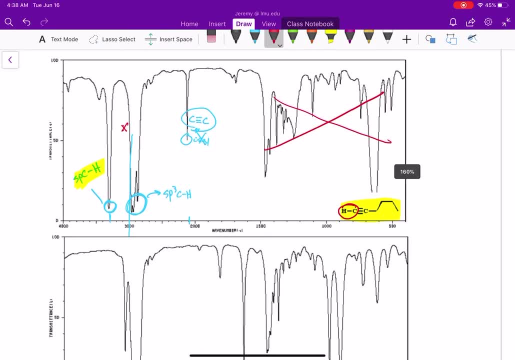 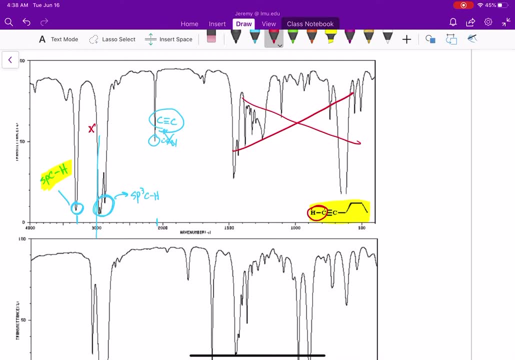 All right, Now a couple questions for you. IR is very useful in determining what functional groups we have, So here we can clearly draw the conclusion that we have a terminal alkyne- Okay. What we can't tell, though, is how many alkynes we have or how many SP3 carbons we have. 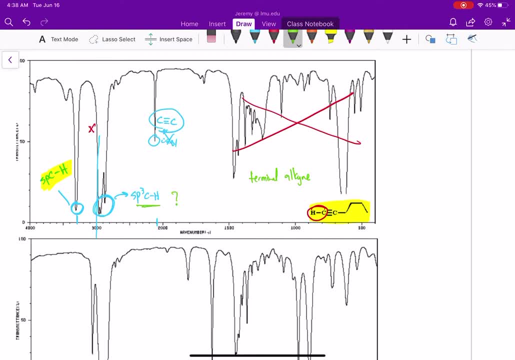 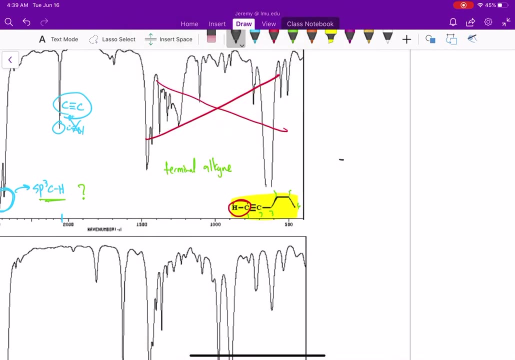 It never tells us the amount, Just that it's present, All right. So here we have one, two, three, four, five, six. This is one hexine, Right. What would the spectrum look like if we had octyne? 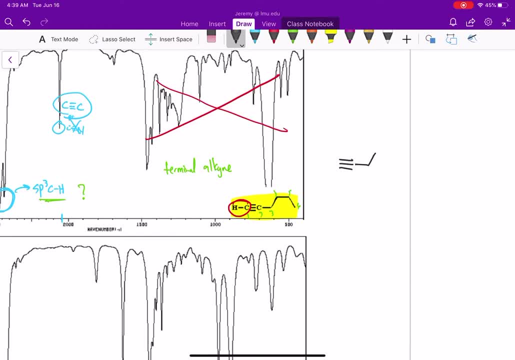 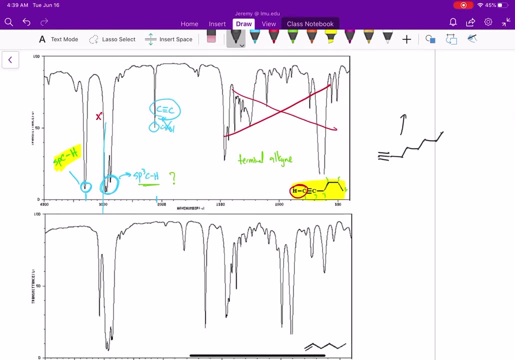 One, two, three, four, five, six, seven, eight. One, two, three, four, five, six, seven, eight. What would our spectrum look like if we had one octyne? It would look exactly the same. 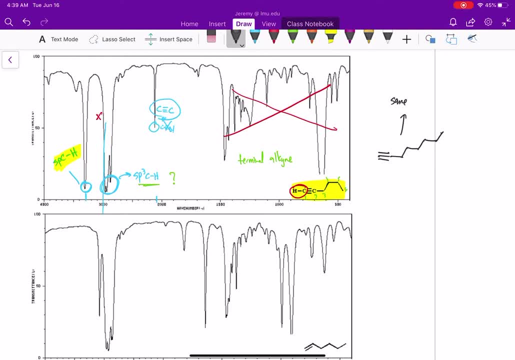 Okay, Our peaks don't tell us how many of the functional groups we have, how many atoms. It doesn't tell us how many carbon-hydrogen bonds we have, Right? So if I extend this chain longer, I've already got CH bonds here and CH bonds. 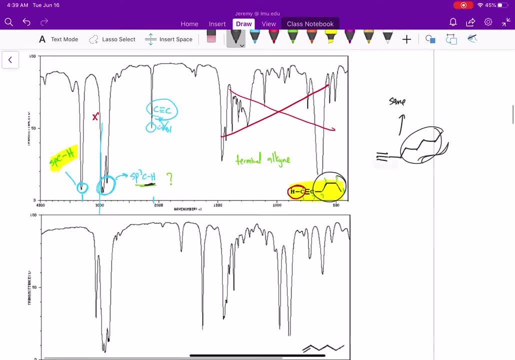 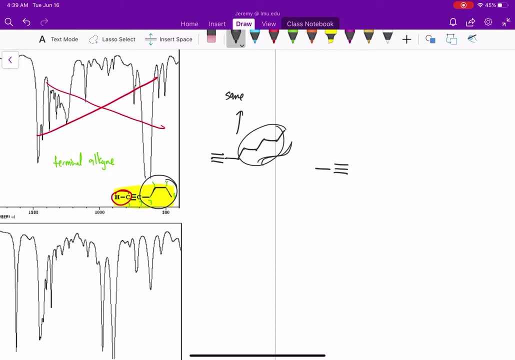 I can't tell the difference there. All right, But what if we had this structure here? What if, instead of having one hexine, we had two hexines? One, two, three, four, five, six? So what if we had this structure? 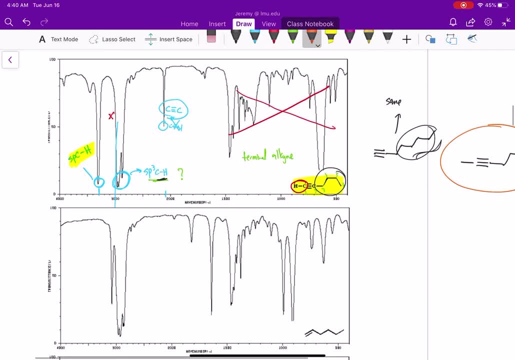 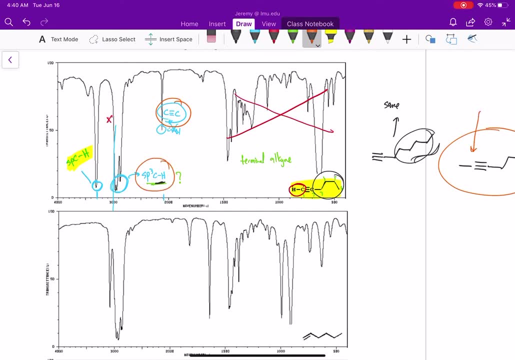 How would this IR spectrum change? Well, we'd still have our carbon-carbon triple bond, We'd still have our sp3C2Hs, But this is no longer a terminal alkyne Right. This is a methyl group, a carbon. 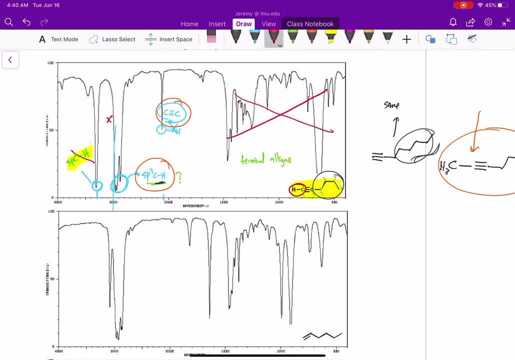 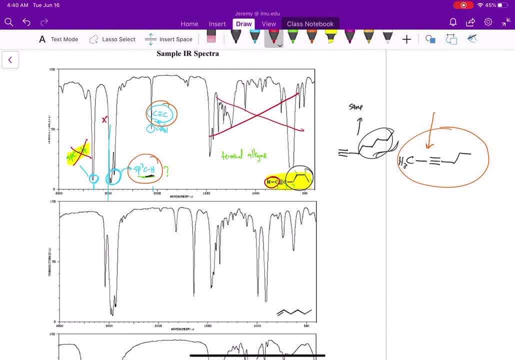 We don't have. We don't have an spC2H bond, So two hexines would not have this peak here. This peak would be gone. It would just be a straight line across. All right, Let's continue on. Let's look at our next structure here. 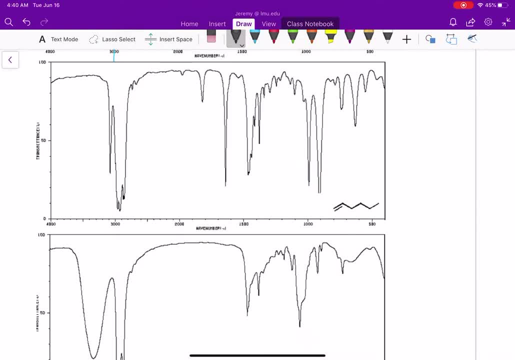 Here we have an alkene, Right. So let's analyze our structure, our spectrum. Nothing in zone one. I get to zone two, Right, I'd like to draw in my 3000 line. So here I can see I have a peak at about 3100. 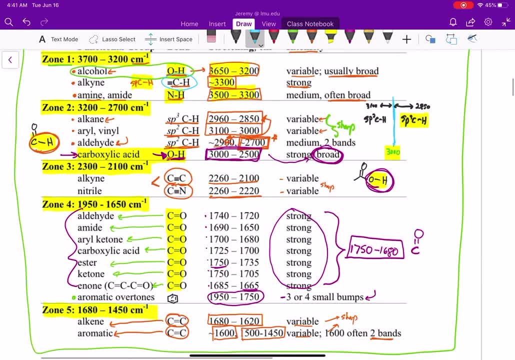 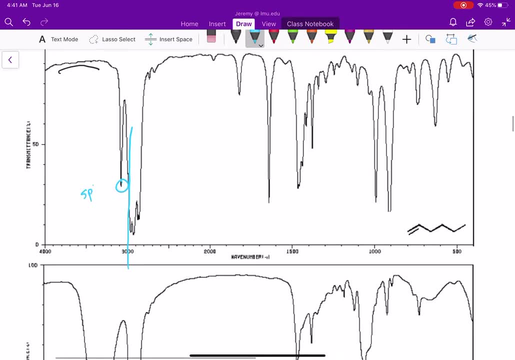 Right Again. we always want to go back. refer to our table. What do I have when I have something to the left of my 3000 line Right? This is going to be an sp2 carbon to H bond Right. 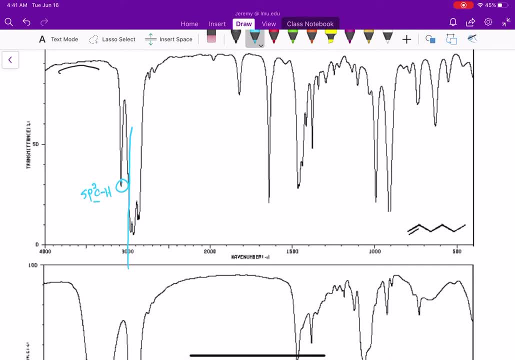 And I'm representing a bond- I always have to draw two atoms Right. It's an sp2, carbon to H. I have a bunch of peaks to the right of that between 3000 and 2850.. These correspond to sp3 C to H bonds. 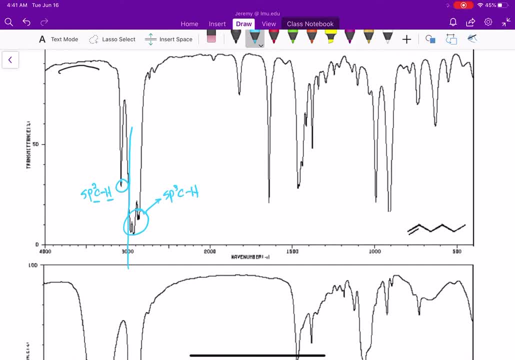 Okay, As I come across, sometimes you'll see small peaks. Right, This is a small peak. We're basically going to ignore it, But there is a large peak here. That's at about, let's say, 1620 or so. 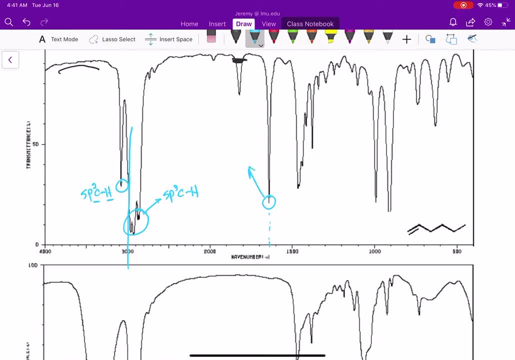 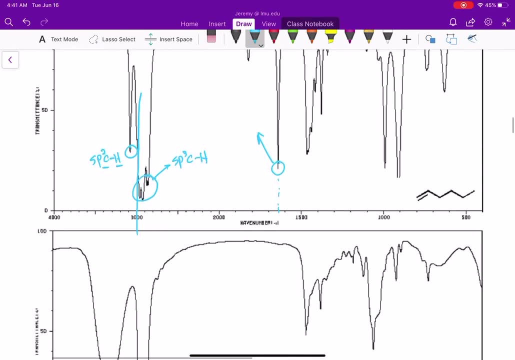 Right 1630.. What does that correspond to? That is in our zone five here Right, And that corresponds to a carbon-carbon double bond. All right, So clearly what we can see here right, is we have some sort of alkene. 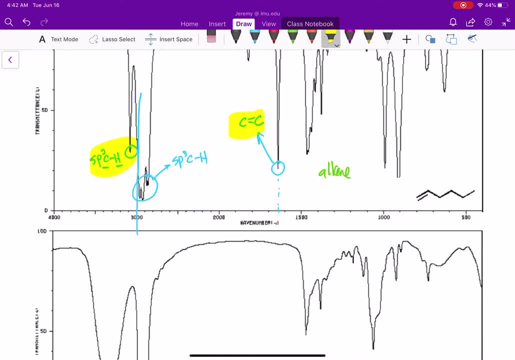 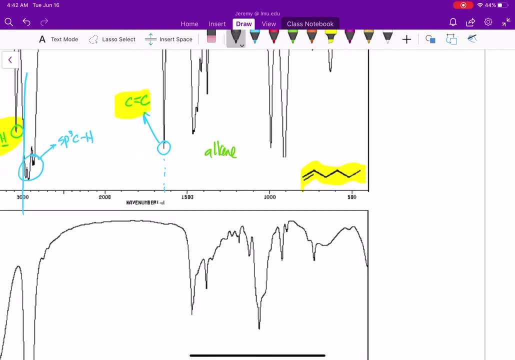 We have an alkene, All right, And that makes sense with this structure here. Now again, from the IR we can't tell what alkene we have. So this same spectrum could fit this molecule here. It could fit this molecule here. 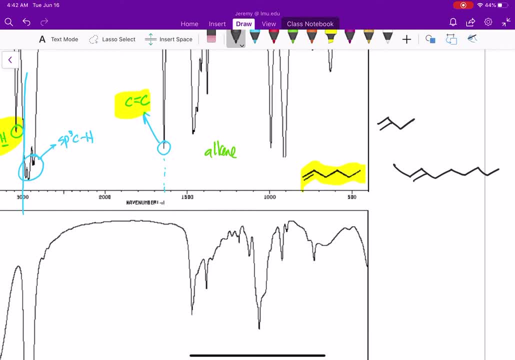 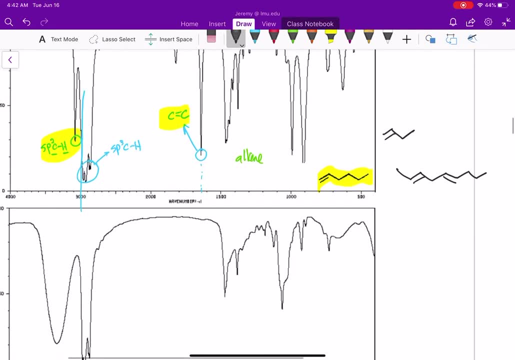 Right. So we have to be aware that it's not going to tell us how many we have. You could have two alkenes. The spectrum is going to look very, very similar. So, in understanding the basics of IR spectroscopy, right. 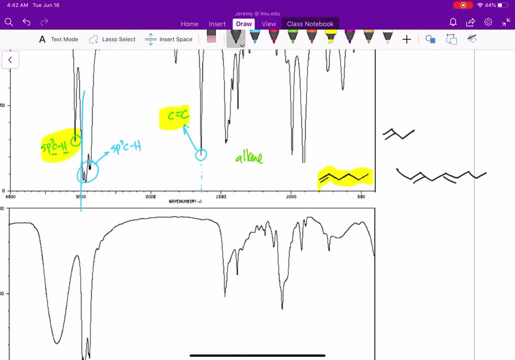 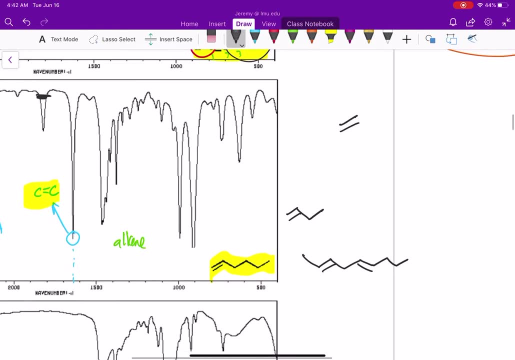 we really need to understand that. it doesn't tell us how many of those functional groups we have, just that we have them. Again, let's do another thought experiment. What if I had this structure here? What if I had this alkene? 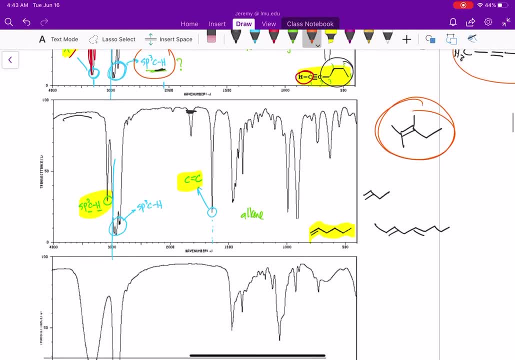 How would the spectrum change? Right, We'd still have our carbon-carbon double bond, We'd still have sp3c to h's. But what we should notice here right, is here we have methyls. This is a tetra-substituted alkene. 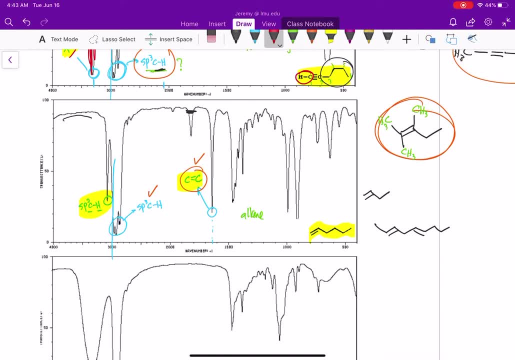 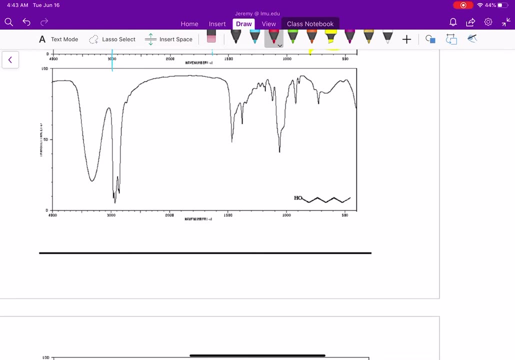 which means there are no sp2c to h's. So the IR spectrum of this alkene that's tetra-substituted will look very similar, but that peak would be gone. We wouldn't see that peak. All right, Looking at our next structure here. 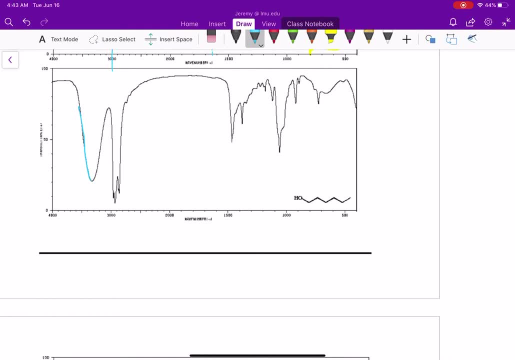 right in zone 1, now we see a big broad peak here in zone 1.. So that's clearly going to be an OH, right, or an NH, Okay, And we'll see NHs a little later. But when you have a nice big broad peak here, 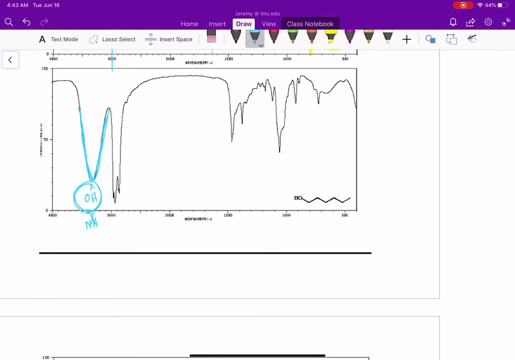 that's always going to be an OH of an alcohol. We get to zone 2.. We draw our 3000 line. nothing to the left of it, A bunch of peaks between 3000 and 2850.. We're generally always going to see these. 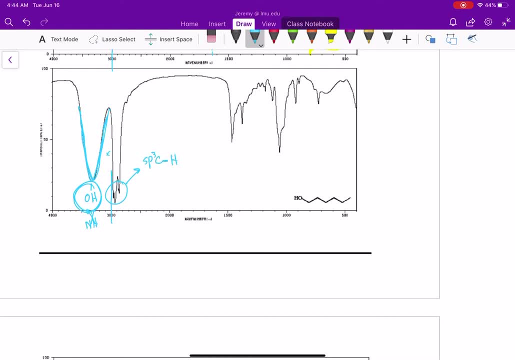 These are sp3, carbon to hydrogen bonds. Nothing in zone 3, nothing in zone 4.. Once we get to our fingerprint region, we can generally ignore that. So what does this tell us? right, This tells us that we have an alcohol. 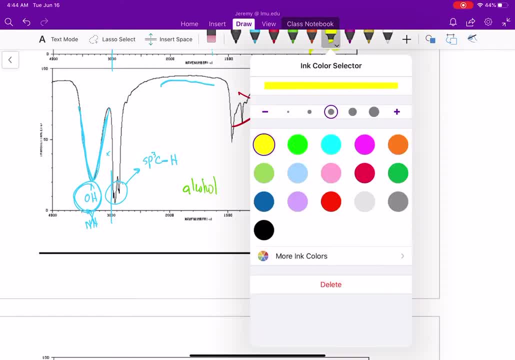 Okay, We have an alcohol here And we can see that functional group in the structure. Again, this alcohol could be lots of things. It could be propanol. Right, It could be cyclohexanol. There's a lot of different molecules that can have a very similar IR spectrum. 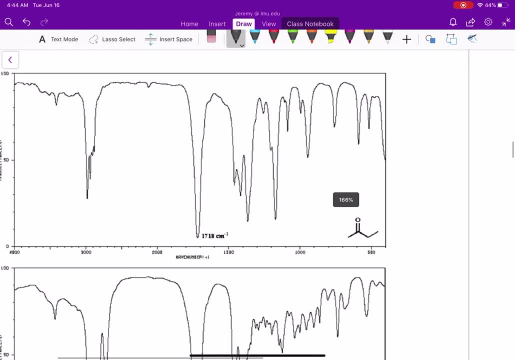 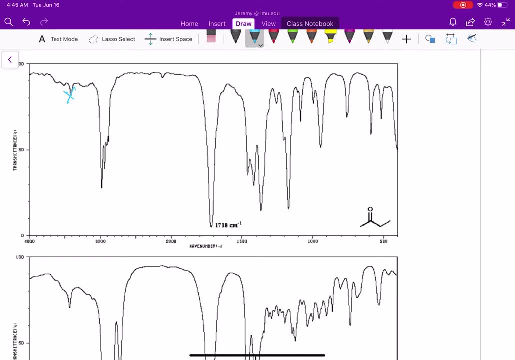 Okay, next we'll start looking at some carbonyl peaks. So when we do our analysis here, we have nothing in zone 1.. We get to zone 2.. We draw our 3000 line. We have a few peaks here. 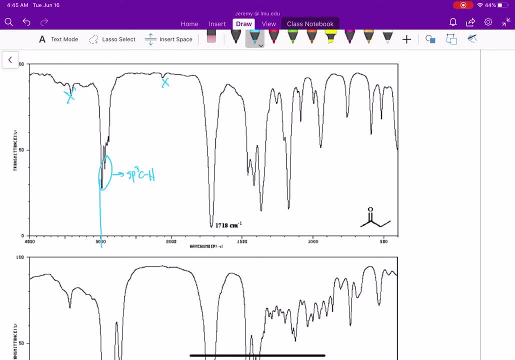 These are sp3s, These are sp3c2hs. Nothing in zone 3.. We get to zone 4 here. Now we have a really large peak in zone 4.. That is our carbonyl. That is our carbonyl at 1718.. 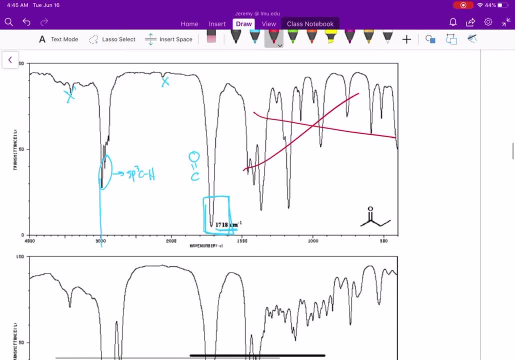 Alright, Once we get to our fingerprint region, we can kind of ignore this. So in this molecule we know we have a carbonyl, Alright, And this turns out to be a ketone- Alright. One thing to notice, right with this table. 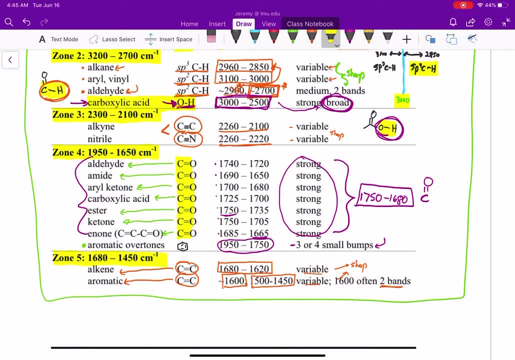 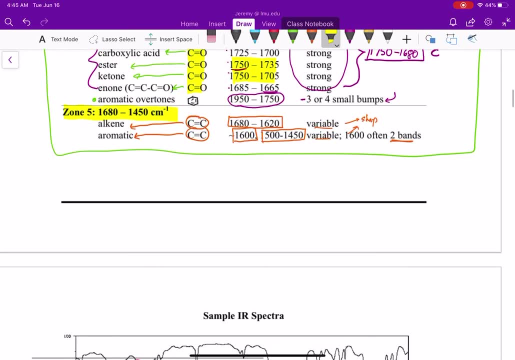 if you look at our ketones, they're 1750 to 1705.. Right Generally the same as an ester. So it's hard to tell the difference between an ester and a ketone at this basic level. But there's other ways to determine those differences. 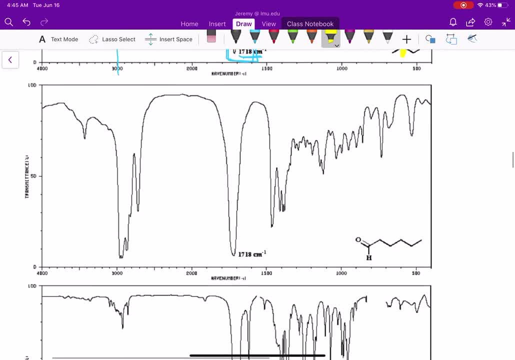 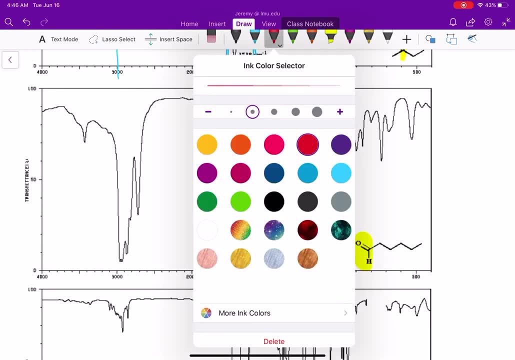 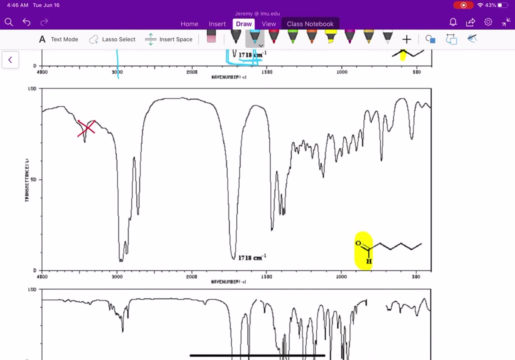 Okay, Alright, so that's what a ketone looks like. Next, we have a functional group here. We have an aldehyde Here. we can definitely distinguish this As we go through zone 1, tiny peak: we ignore. We look at zone 2.. 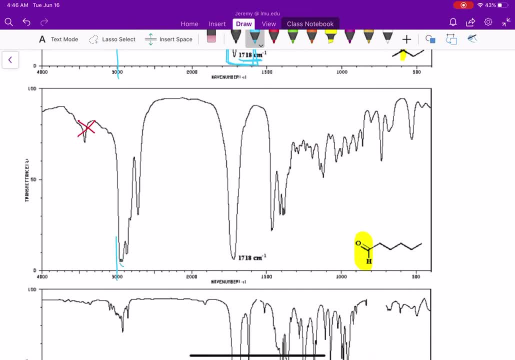 I draw my 3000 line. I circle my peaks from 2850 to 3000.. Those correspond to sp3c, to h's. And now I have this other peak, way out by itself at about 2700.. What is that? 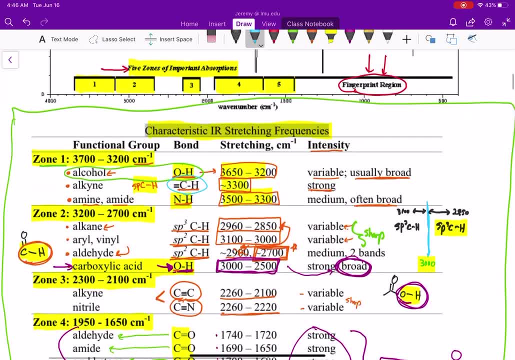 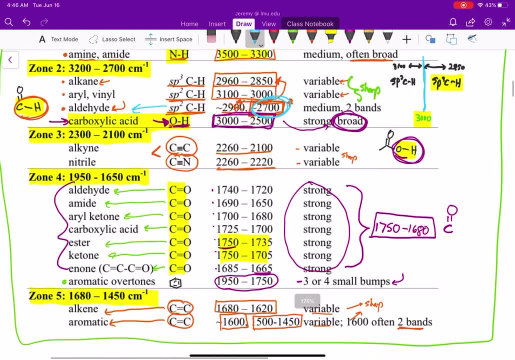 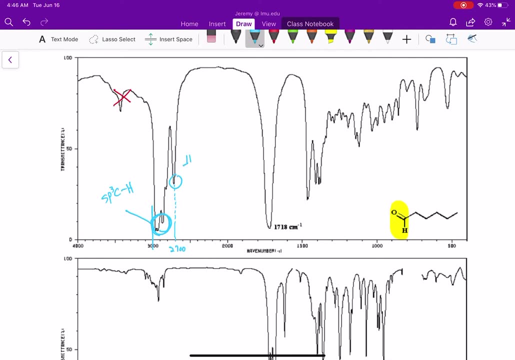 There is only one peak that absorbs, at 2700.. And what is it? 2700 is my aldehyde. Okay, So this peak here at 2700, this is our aldehyde But specifically, it is this bond here, It's the c to h bond. 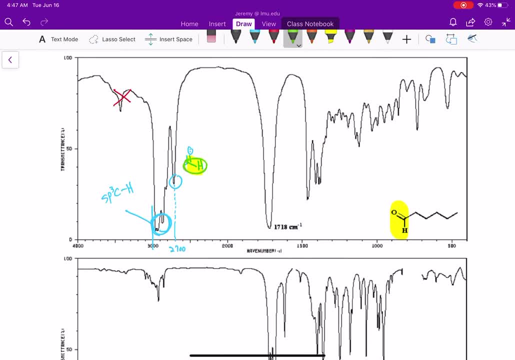 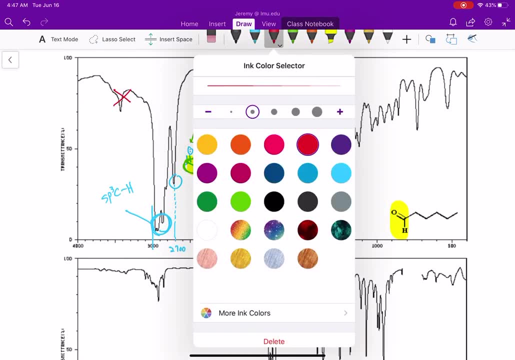 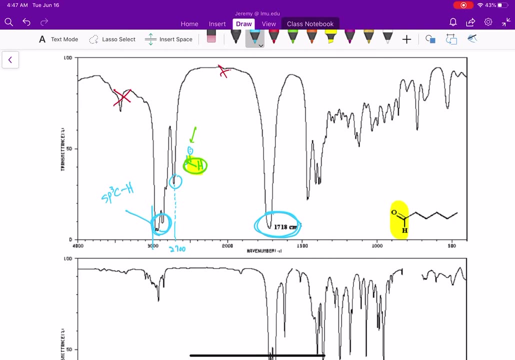 Alright, Okay, Now when you draw an aldehyde, what else does an aldehyde have? It has a carbonyl. Where does that show up? Right, Nothing in zone 3.. But in zone 4, we've got a huge peak at 1718. 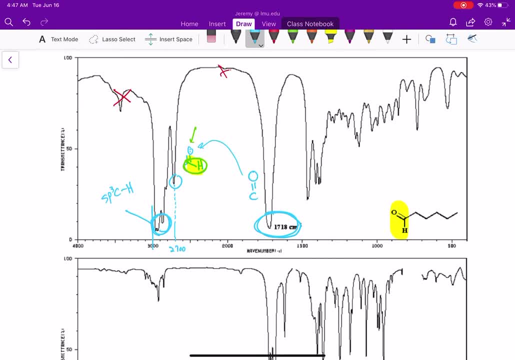 That is the carbonyl of the aldehyde. So you see, when you have an aldehyde you have two distinctive peaks. You've got your 2700, your sp2c to h, And then you have the c double bond O at 1718. 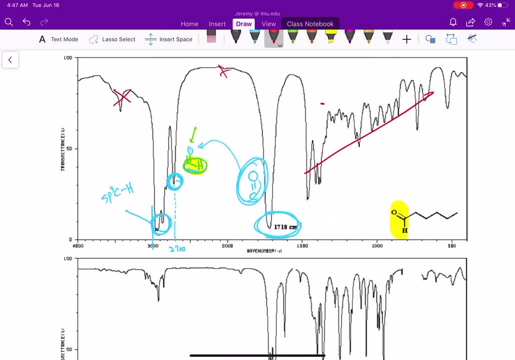 Okay, We get down to the fingerprint region. We can basically ignore that. This peak here is important because it tells us we have an aldehyde Again. we don't know how many carbons we have here. We definitely have some because we have sp3 carbons. 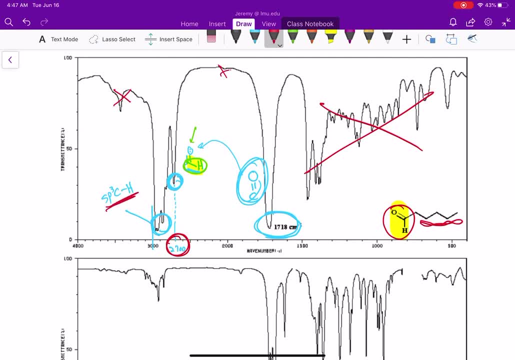 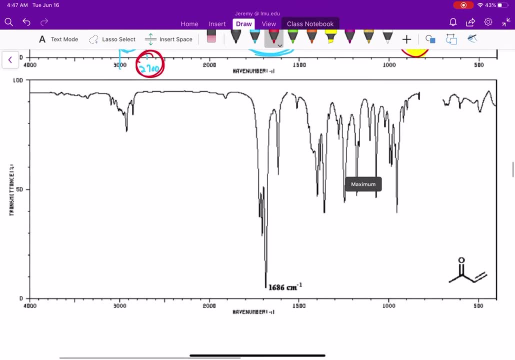 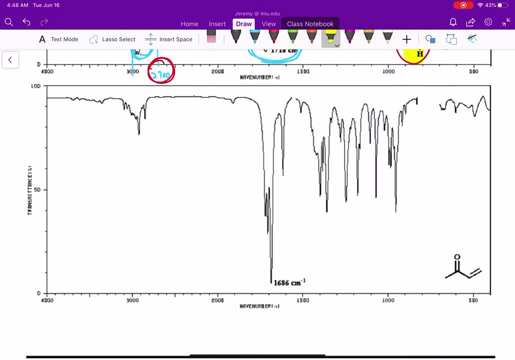 but we don't know exactly how many. Again, the purpose of IR is to tell us: do we have that functional group or not? Alright. Next example: here we have an enone. We have a conjugated ketone. Okay, So we have a conjugated alkene and ketone. 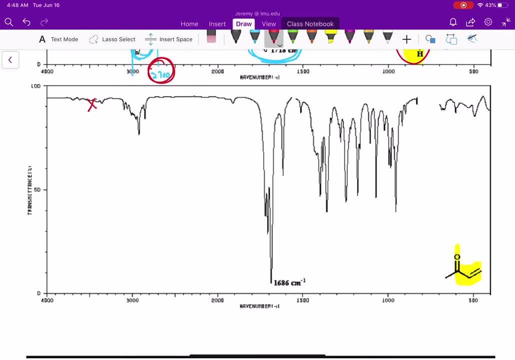 We get into zone 1.. Nothing here. Zone 2. Now we do have some peaks Right. So if I draw in my 3000 line here Right We can clearly see we have some peaks to the left and the right. 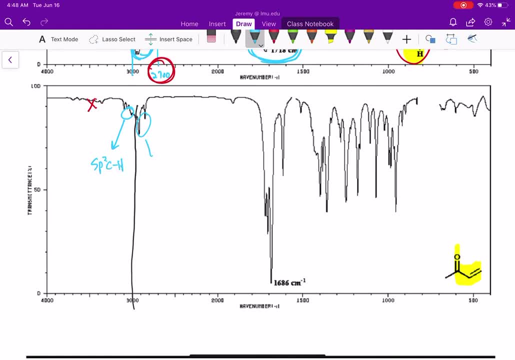 They are small Right, And they are there. So these correspond to our sp2 C to H's between 3000 and 3100.. And the sp3 C to H's between 3000 and 2850.. Nothing in zone 3.. 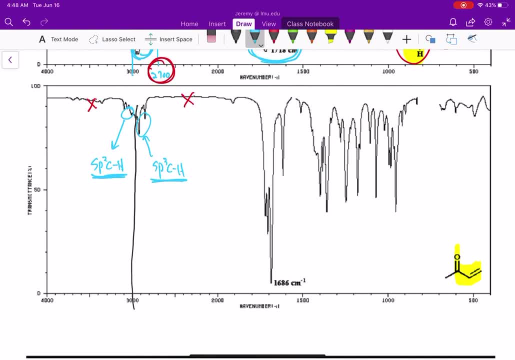 Right, And now we get into our zone 4.. Alright, What we can see here is we have a big bunch of peaks here at 1686.. That's still in zone 4.. That is our carbonyl Right, Because this is kind of low. 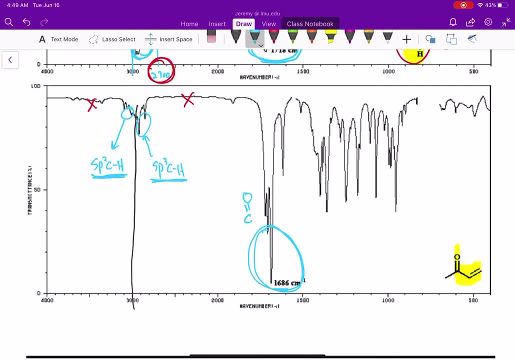 it tells us that we most likely have a conjugated system. And then here we see our peak at about 1600.. That's our C, double bond C. Okay, So generally in my class, what I'm going to do is, anytime I give you a carbonyl. 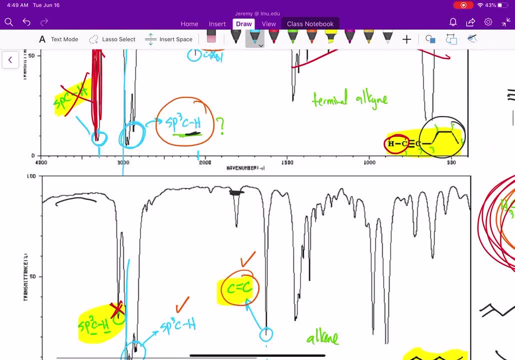 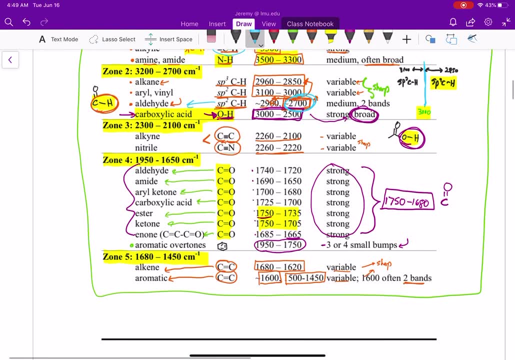 Right, I'm generally going to give you carbonyls that don't overlap into into zone 5.. So my carbonyl peaks here. I'm going to give you things that I'm not going to go all the way down to 1665.. 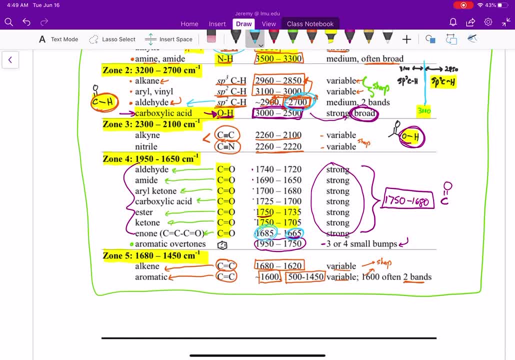 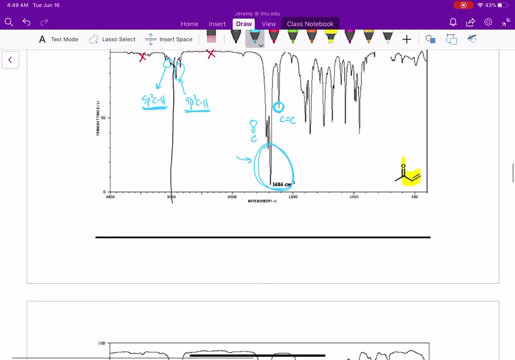 Right, It'll be closer to 1685.. It'll be above 1680.. So you can clearly see that that carbonyl peak is in zone 4.. And if you look at that peak here, that's clearly in zone 4. 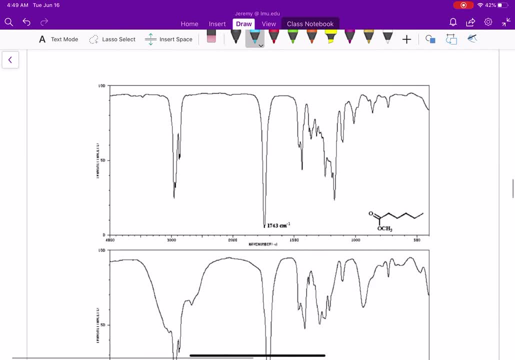 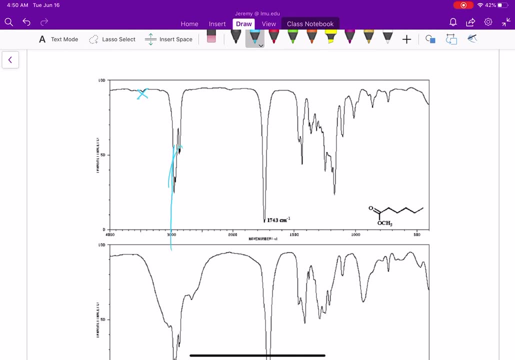 and not in zone 5.. Alright, Next spectrum is the spectrum here. Nothing in zone 1. Right We draw on our 3000 line A few peaks to the right of it. Again, those are SP3 C to H's. 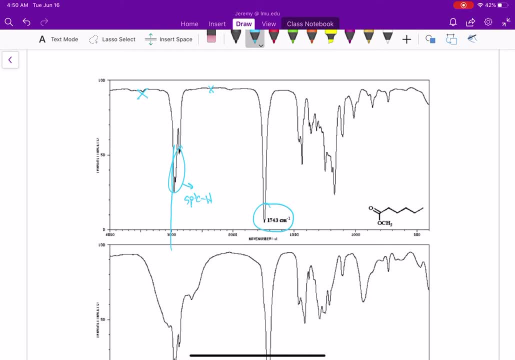 Nothing in zone 3.. Zone 4: we have a huge peak here. That is our carbonyl 1740.. We can basically ignore our fingerprint region here. Again, here, this is an ester. Okay, And what we talked about here. 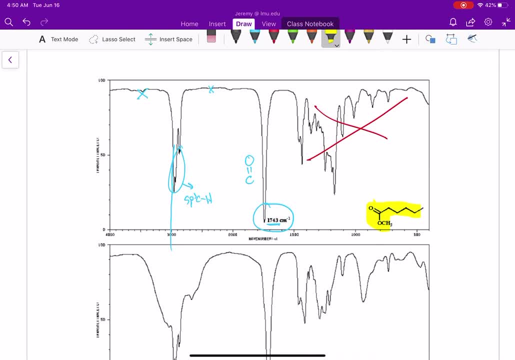 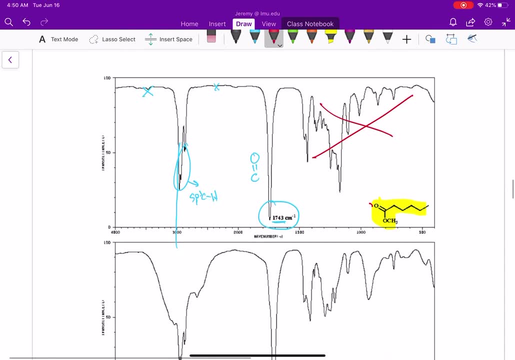 esters and ketones are quite similar, So I'm going to have to give you some extra information to determine whether you have an ester or a ketone Right. But what you'll notice with an ester is you generally have two O's. 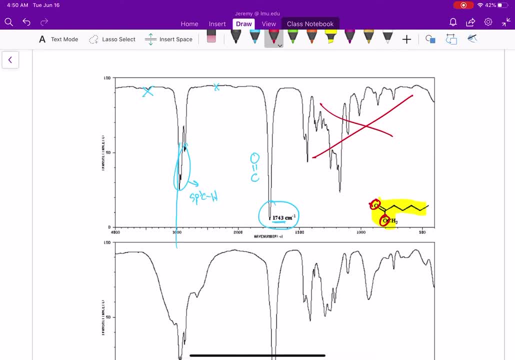 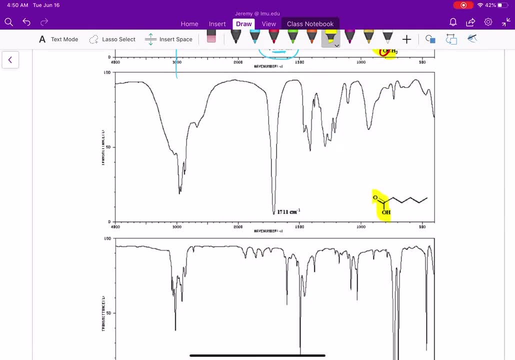 Right, You have two O's. The ketone might just have one. Alright, Our next example we'll see is a carboxylic acid. These have very distinct peaks. So if I look in zone 1, I don't have anything separate in zone 1.. 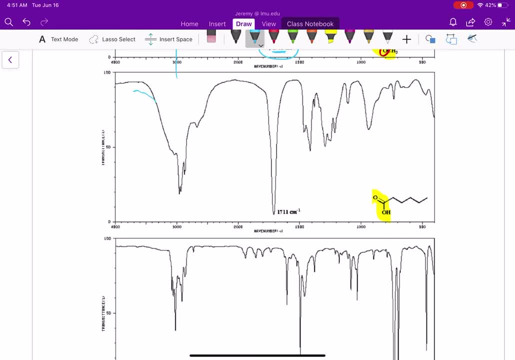 Right. But if I draw my 3000 line I can clearly see some peaks to the right of that. That's my SP3 C to H. But in the background here I can see this big broad peak, And that big broad peak here is in zone 2.. 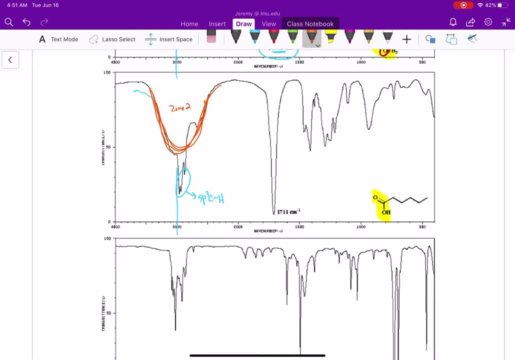 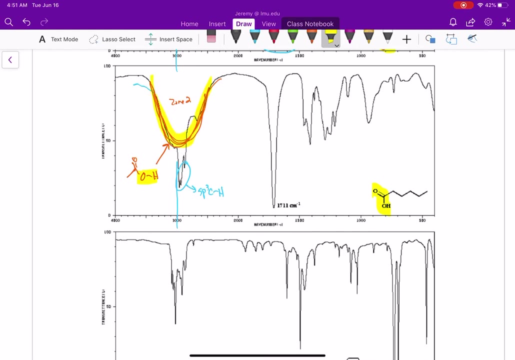 Right. So when we have this big, broad peak here and it's in zone 2, that is the OH of a carbonyl Carboxylic acid. Okay, That's the OH. So when you have this big, broad peak in zone 2, 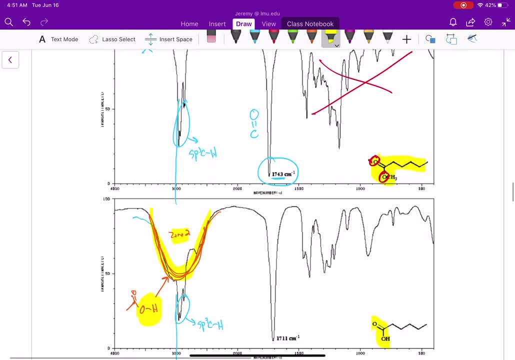 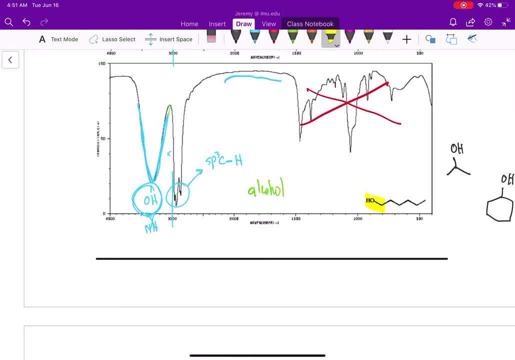 that tells you you have your OH of a carboxylic acid. Let's review and look at what an alcohol looks like. Remember the OH of an alcohol was clearly in zone 1.. Okay, So alcohols are clearly in zone 1.. 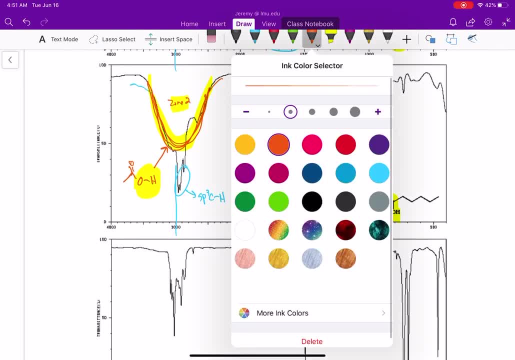 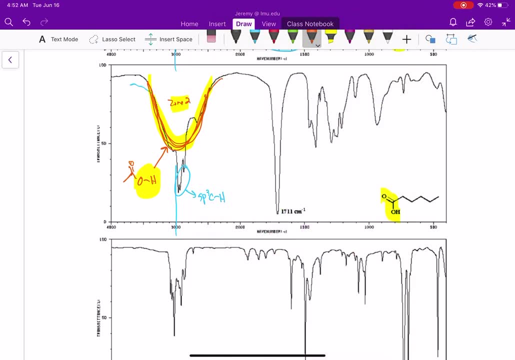 Carboxylic acids really expand all the way out through zone 2. And that's how you can tell you have a carboxylic acid. Nothing in zone 3.. We get to zone 4.. Of course we have that large carbonyl peak. 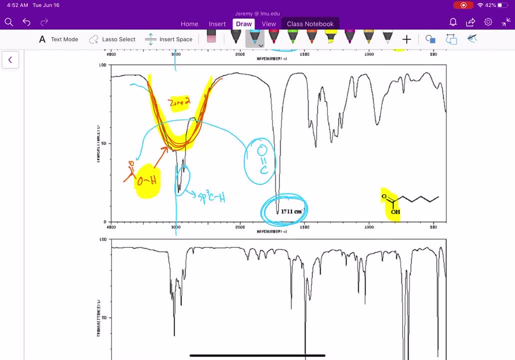 So this is the carbonyl peak of the carboxylic acid. Carboxylic acid is going to have these two big peaks: The OH in zone 2 and your carbonyl. Okay, We can ignore everything below 1500. 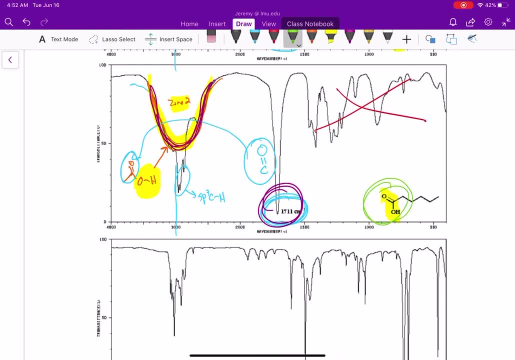 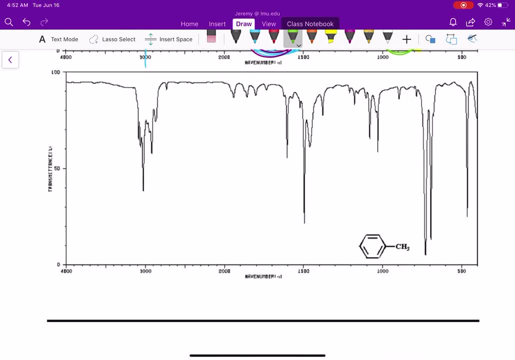 And clearly we have a carboxylic acid, Carboxylic acid. Alright, The next spectrum that we can look at here, And I think this is the last one we're going to look at, Let's identify this: Nothing in zone 1.. 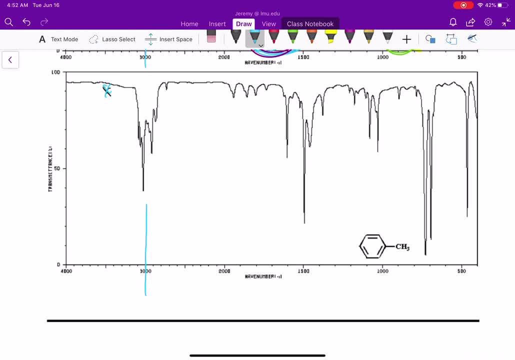 Right Zone 2.. We can draw in our 3000 line. We see we have some peaks to the left of that Between 3100 and 3000.. Those are clearly sp2 C to H bonds. We have peaks to the right of that. 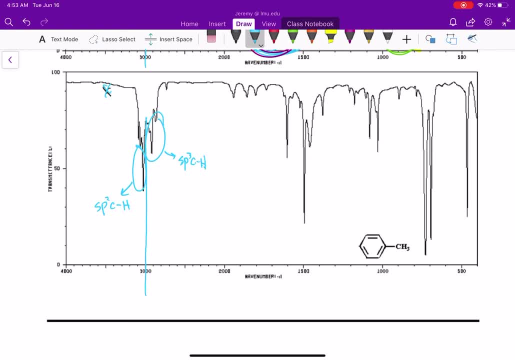 Those are sp3 C to Hs. Nothing in zone 3.. In zone 4. We see 3 or 4 small bumps Right. Those are what our aromatic overtones look like. That's a really good indicator, of course, that you have an aromatic ring. 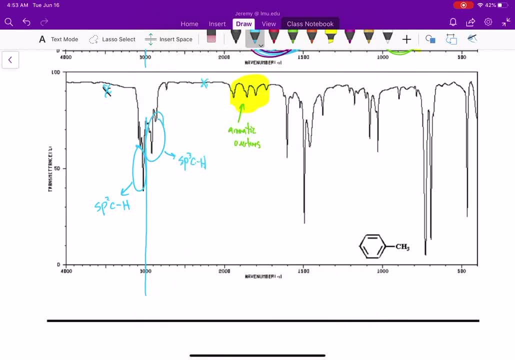 Alright. And then our last peak. we can see we have a peak here, Right, And that's our C double bond C of our double bond Right, And there's generally a second one of those, Alright, And we can kind of ignore everything below 1450.. 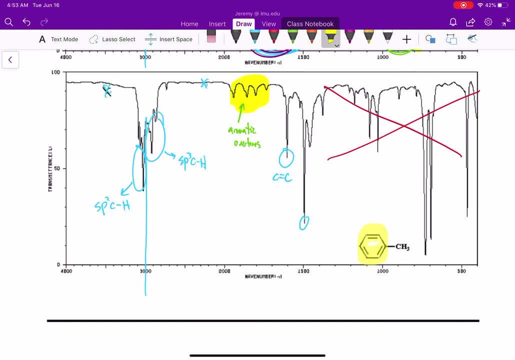 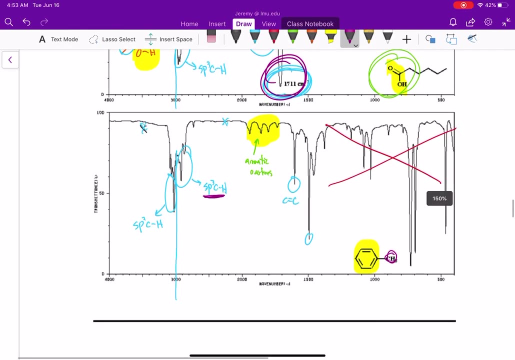 Clearly here. we know we have an aromatic ring of some kind, We have a benzene ring Right, And because we have some sp3 C to Hs, we have to have some sort of alkyl group coming off. that Alright. So that is basically kind of an introduction to infrared spectroscopy. 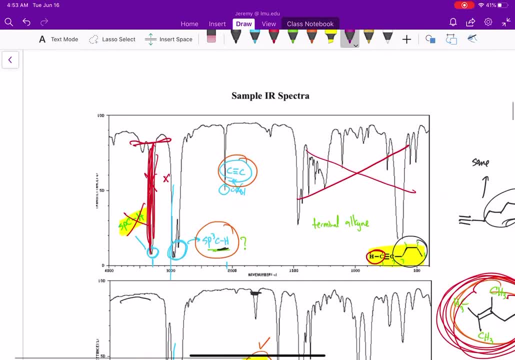 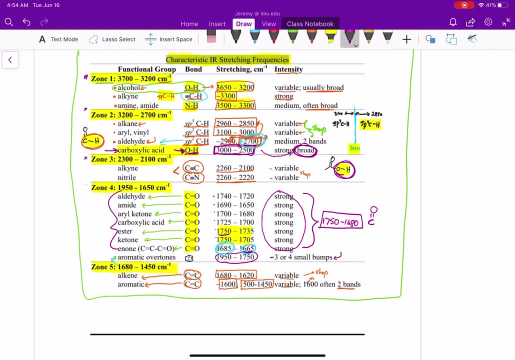 It's important that you know the table Right. So it's important for us to know this table. Analyze this by the basic zones Right. And then we saw examples of the key functional groups we need to look at.